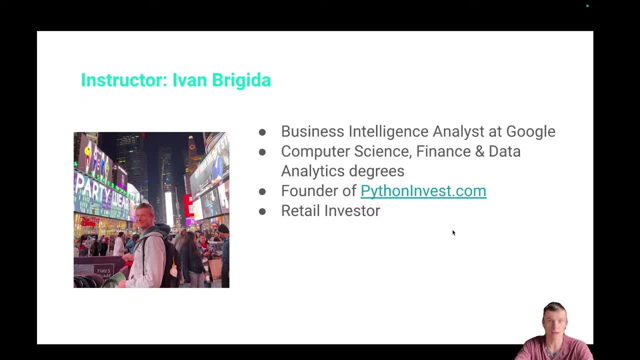 For those who don't know me, I'm Ivan Brigida. I worked for about 10 years at Google as a business intelligence analyst. I have a computer science degree and another degree on finance and data analysis. I founded pythoninvestcom project about three years ago, where I wrote different analytical 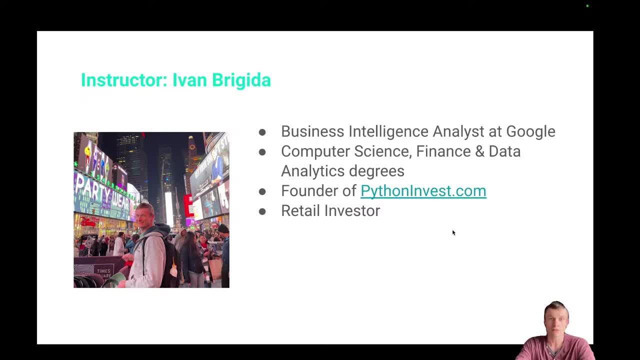 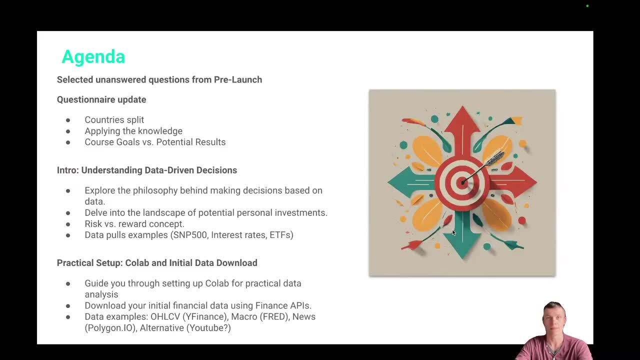 articles and long reads, And also about that time I started to do trading as a retail investor. Today we will cover these sections. First I'll talk about trading. I'll answer some of the questions that we didn't have time to answer during the prelaunch. 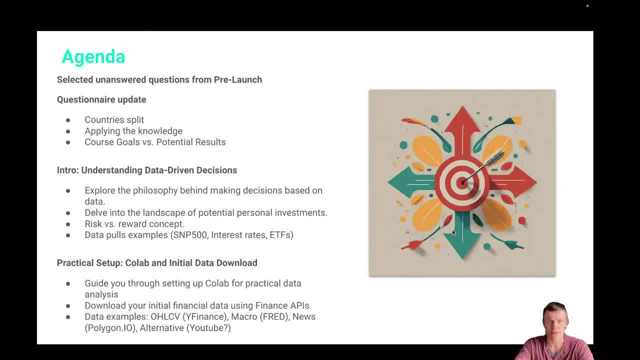 session. Then I will update questionnaire results. Next we will talk about introduction and try to understand data driven decisions. That's why that's we will try to explore the philosophy of a trader and investor will see landscape. We'll talk about the landscape of potential personal investments as a retail investor. 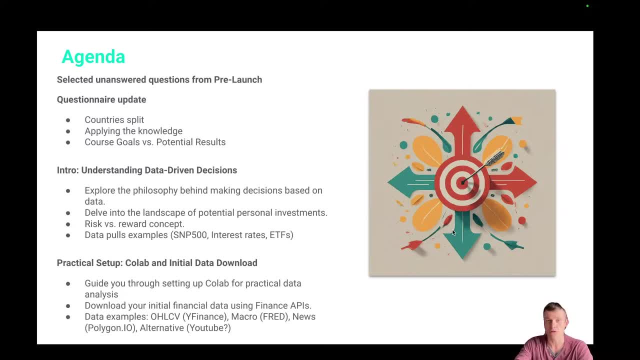 We'll talk about risk versus reward concept and I'll show you some of the data pools. Next we'll switch to call up and to different data sources which you might use for your projects and for your- for your- homeworks, Just as a reminder. 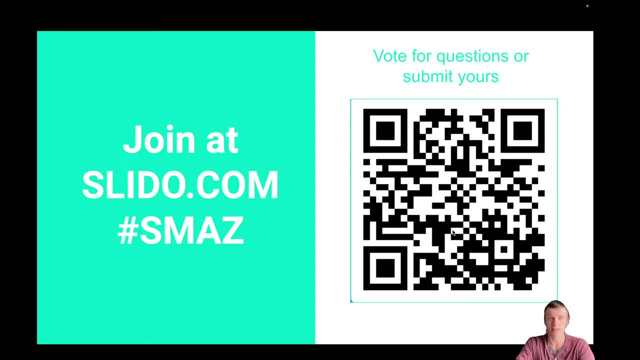 You, Please, Please, Call up to the slides on And at this hashtag, as am a set, and ask questions. vote for questions that are related to the content. We won't be able to answer To your life questions on YouTube, But I will try to to check all questions that you ask in slide or in telegram or in slack. 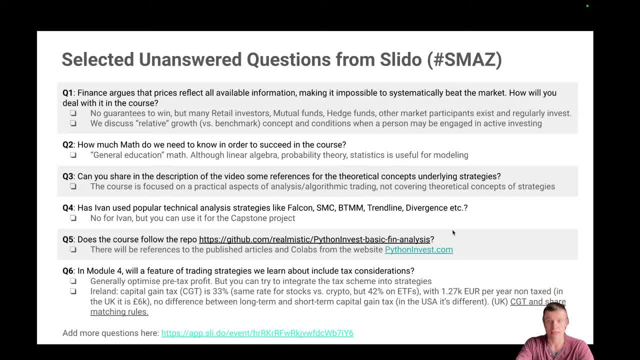 Here Are few questions that I didn't answer previous time. First, finance argues that prices reflect all the available information, making it impossible to systematically beat the market. How will you deal with it in the course? I know about it, but of course there are no guarantees. 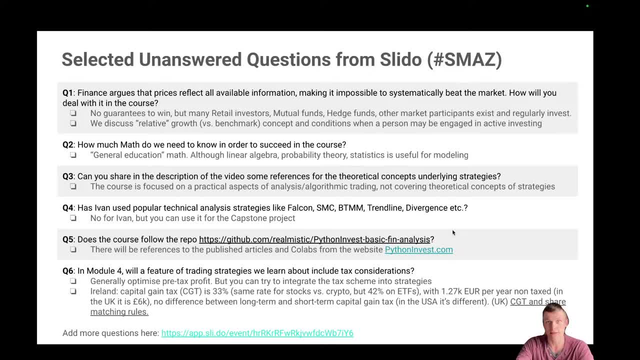 to win or to beat the market, But there are many retail investors, mutual funds, hedge funds and other financial organizations who regularly invest and participate in this activity. So it's up to you whether you want to participate or whether you want to try and do risk management when you see no profits. 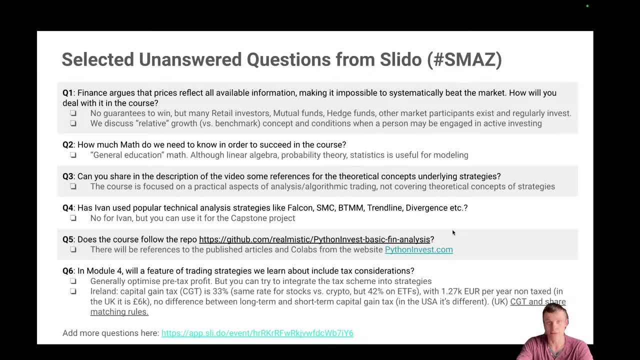 Second thing, we will discuss the concept of a relative growth versus some benchmark, and you will need to define a benchmark that you compare yourself against, And we will discuss the conditions when a person should engage or not engage in active investing or trading. Question two: How much math do we need to know in order to succeed in the course? 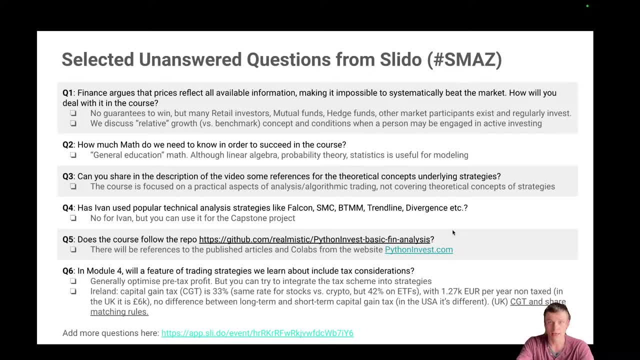 I'd say you don't need to know any advanced math. What you need to know is general education math, Although if you want to do some complex models or complex simulations, linear algebra, probability theory, statistics will be very useful for you. 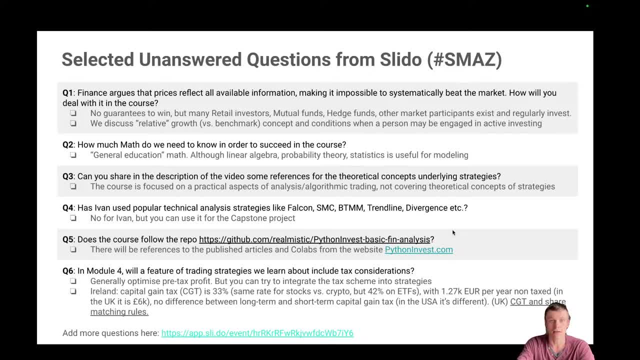 Question three: How can you share in the description of the video some references to the theoretical concepts underlying strategies? I do not cover any theoretical concepts because the breadth of the theoretical concepts of the courses is quite, quite wide. But you can always Google those theoretical concepts. 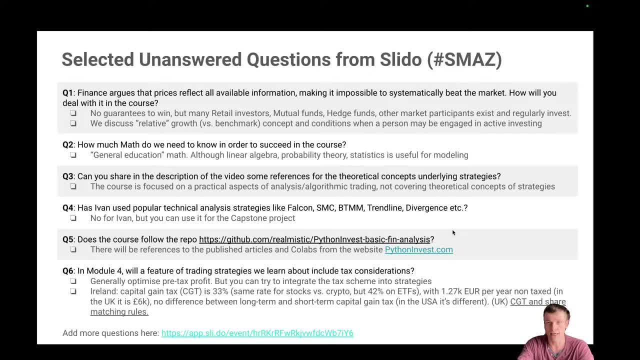 We will focus purely on the practical aspects of analysis, coding, simulation and training. Has Ivan used popular technical analysis strategies like Falcon, SMC, BTMM, Trendline, Divergence, etcetera? I hope not. can't name myself as a technical trader so I do not use these strategies, but I think this is a 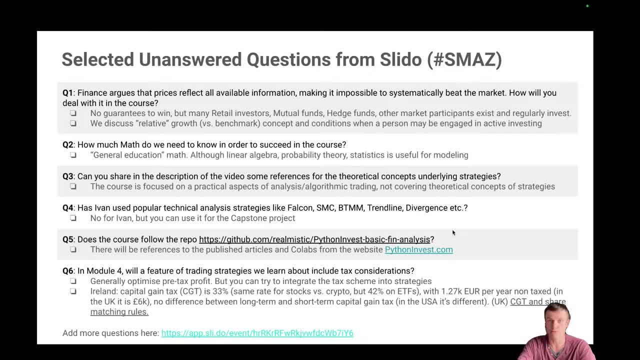 perfect example to use in your capstone project. Does the course follow the repo? python invest: basic finalist analysis? That repo has many collapse from my long reads. I will add links to the articles and to the code where I can, but the course doesn't follow directly this repo. 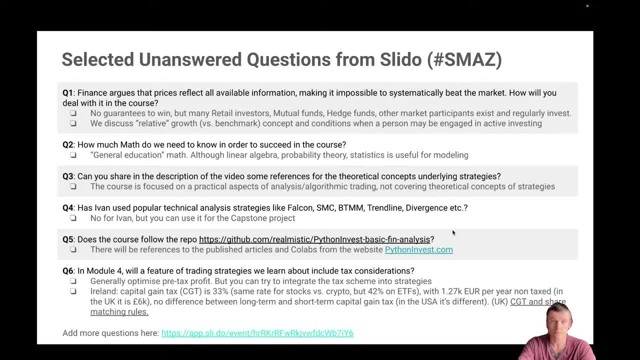 All content is new. it's never published before. Question six In model 4: will a feature of trading strategies we learn about include tax considerations? This is a very interesting question. Generally, I do not use this. I optimize pre-tax profit, but you can try to integrate your tax schemes to their strategies. For example, I read: about capital gain tax, CGT in Ireland and it is 33% on all types of stocks and crypto, but 42% on ETFs. That's why, probably, I'm more incentivized to trade stocks instead of ETFs. Then in Ireland we have 1.27k euro capital gain that is not taxed in a year In the UK it is 6,000 pounds. So you might want to invest and to see the profits that are less than this sum not to be taxed or calculate the tax gains that you might incur. Then we don't have any difference between long-term and short-term capital gain tax compared to the USA. 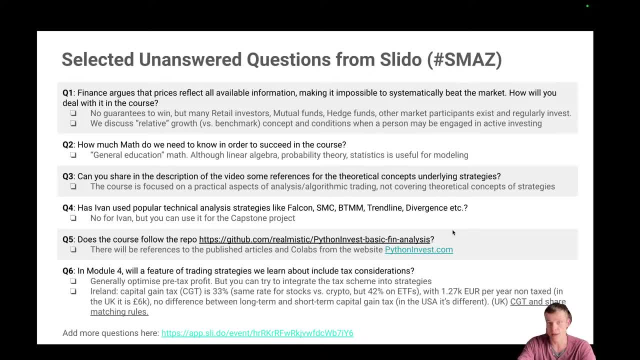 Then, more than that, in the UK there are CGT and share matching rules, which is an interesting thing, which says that if you sold some share and bought it again in less than 30 days, you might pay less taxes. This is also can be used for your strategies, and 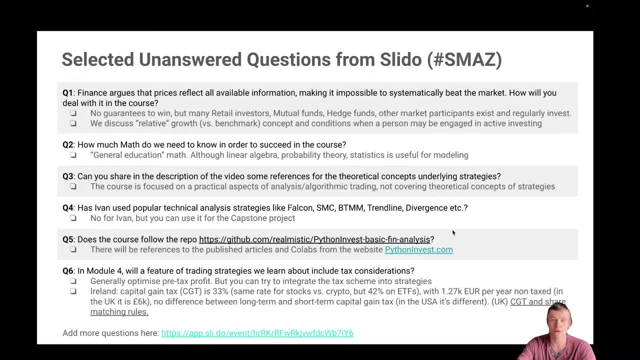 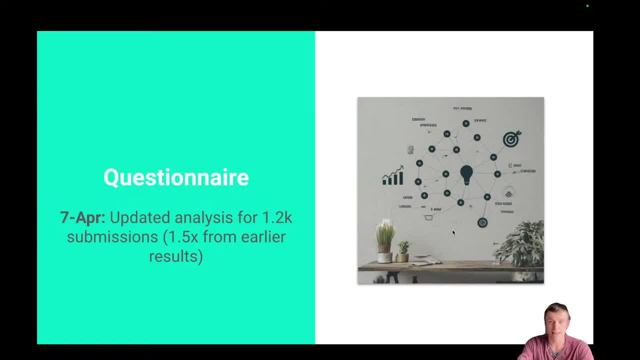 you can try to use this. try to do this and show in your projects. Now let's switch to the questionnaire. I've updated the analysis on the data one week ago. It is about 1,200 submissions, or 50% more people answered to the questions. 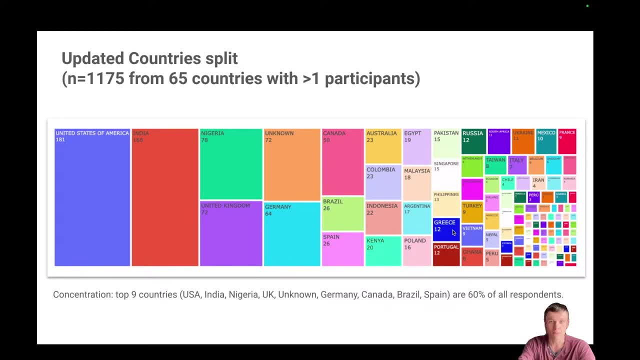 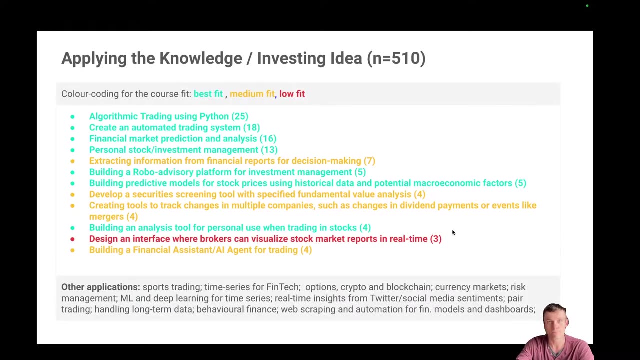 The country split is approximately the same, With the leading countries USA, India, Nigeria, UK, Germany, Canada, Brazil and Spain representing about 60% of total answers. Next, I've updated the analysis using chat GPT API and I asked: 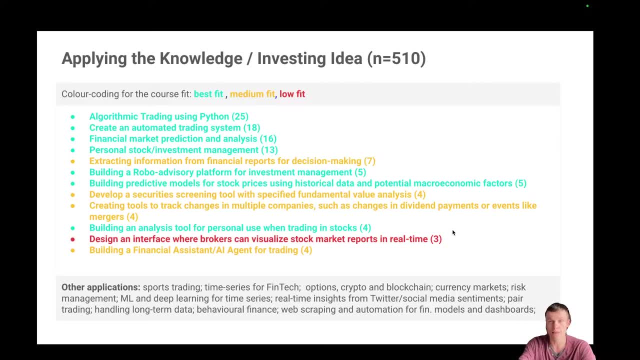 to analyze your responses to the question how you plan to apply the knowledge that you will receive Or what are the investing ideas that you have. Now we have more answers. It is about 500 answers and they color-coded those answers which are best fit, medium fit or low fit for this course. 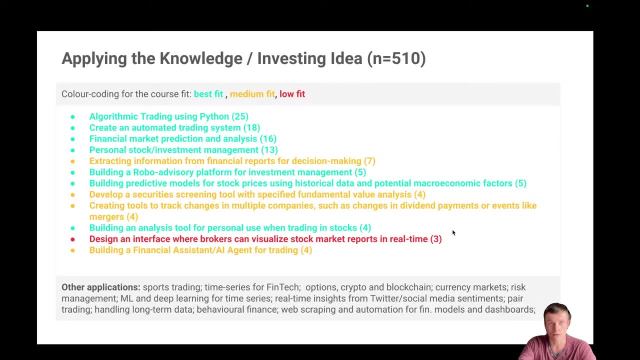 Of course, I'm trying to cover as many aspects as I can about algorithmic trading using Python. We will try to create an automated trading system and we will try to do financial market predictions and analysis. We will always talk about personal stock and investment management as a retail investors. 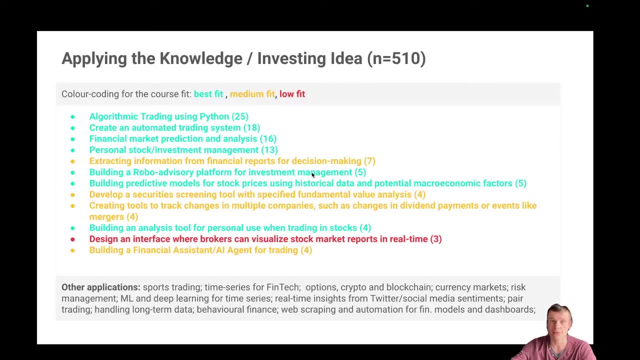 We won't be covering that much information. extract information from financial reports for decision making, Although today we will cover SEC ADGAR data source so you can go and write an algorithm to extract those reports and analyze them somehow. What we're trying to build here it's very close to robo advisory platform. 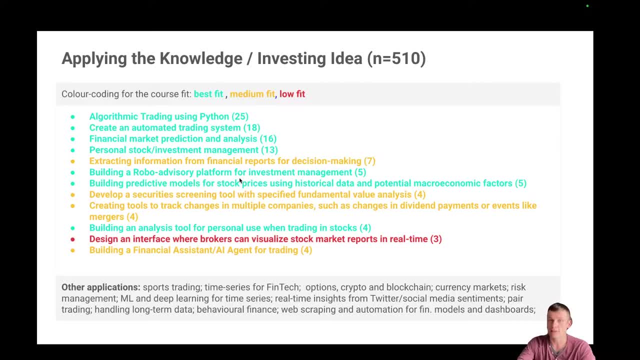 or what current robo advisory platforms offer you. Then we will talk about predictive models for stock prices using historical data and potential macroeconomic factors. We won't go too much into the specifics of machine learning models and different types of them, but I will show you. 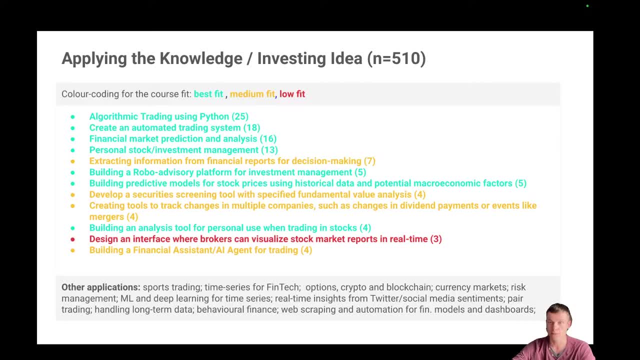 some examples which you can replicate straight away using your data. We won't talk much about how to develop a security screening tool for specified fundamental value analysis, Or how to create a security screening tool for specific fundamental value analysis, Or how to create a security screening tool for specific fundamental value analysis, Or how to create 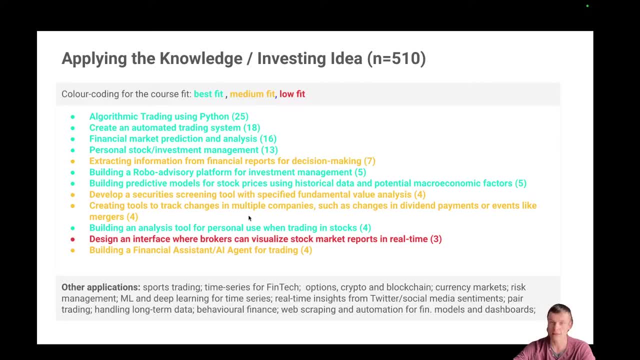 tools to track changes in multiple companies, So you can combine all of that. but it's not about visualization. it's not about web services and product tools for the market. We will try to build the analysis tool or try to build a comprehensive data set for 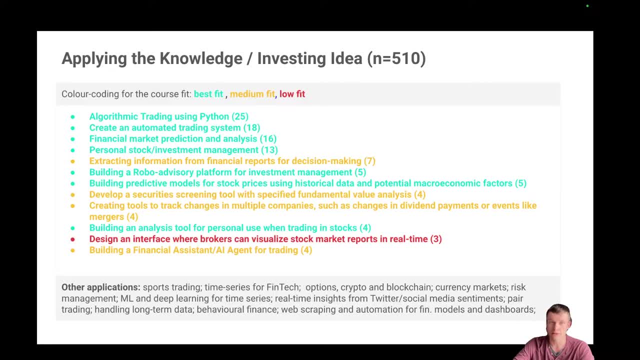 intangible data, that that is used for personal use when you do trading stocks. We won't design an interface where brokers can visualize stock market reports in real time, But probably for someone who is working for a broker it can be very, very useful to understand. 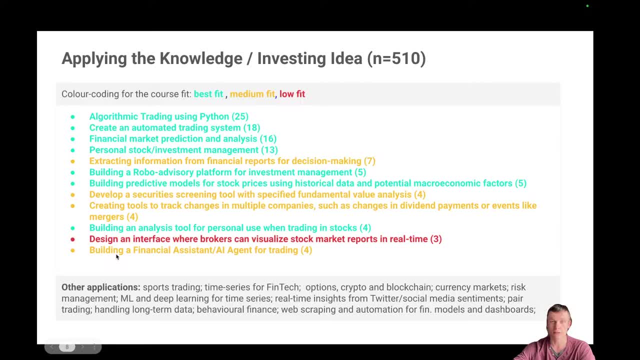 what is needed by the market. We won't build a financial assistant or AI agent for trading. the next steps have been shown in a. in performance analysis saw that Datatox started their or plan to start their new course on LLM and, if any of you can, 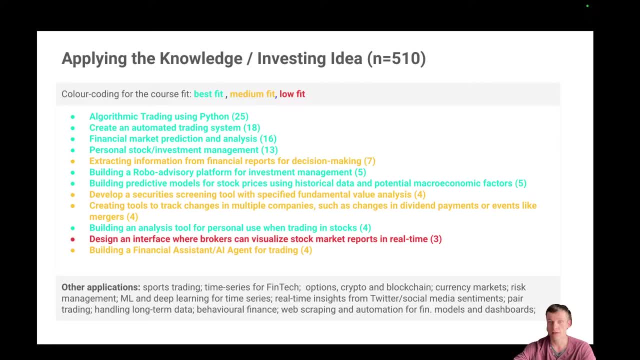 actually build this financial assistant or AI agent. I would be very happy to see this in the projects. There are many other interesting applications like sports trading, time series for fintech options, crypto currency markets, risk management, MLM deep learning, real-time insights. 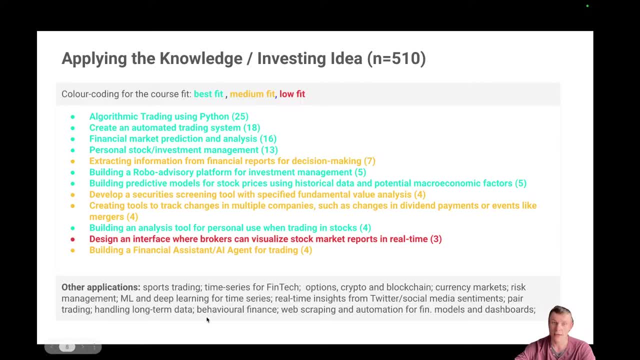 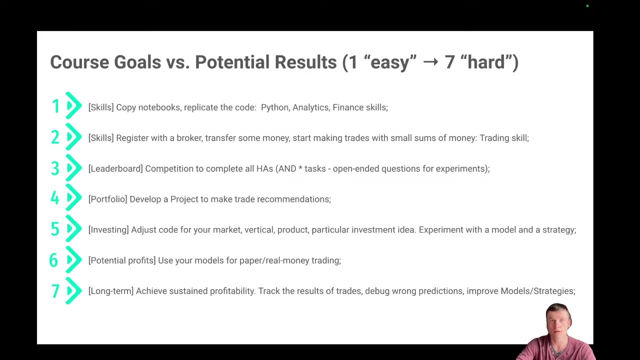 pair trading handling, long-time data, behavioral finance, web scraping and automation mentioned. We will try to cover a wide variety of topics, but probably not all of these topics. On the next slide I tried to categorize the involvement and time spans and goals that you. 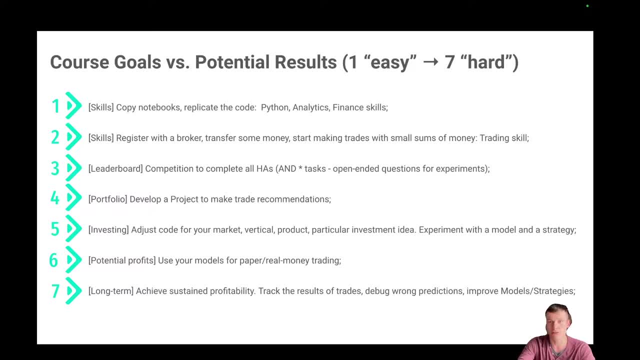 might have when you plan to finish your project. We will start from easy ones, that is, one, two, three, and we will finish with the hard ones, where you need to be fully in the course, so easy you will get, where you will obtain new skills. you can copy notebooks, replicate the code. it will be python, analytics, financial. 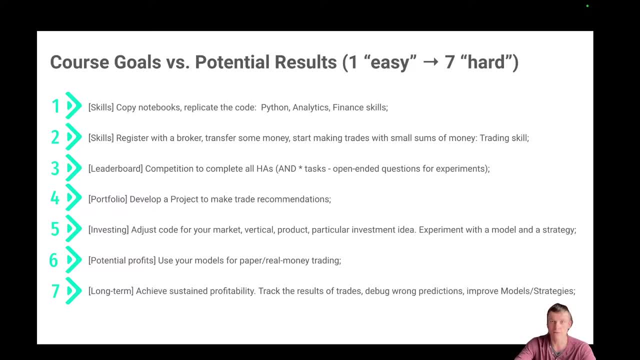 skills, automation skills- very useful skills for your future or existing jobs. Second, you can register with the broker. I saw that there were not many people who do active trading or who do trading with real money at all, so it can be a first step that it's not that complicated and, as a result, you can get a trading skill. 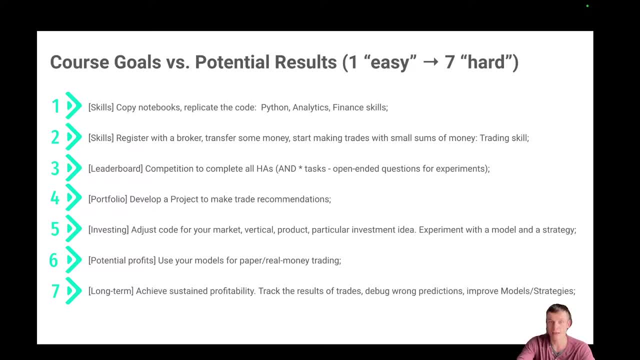 Third, we all love to compete, so there will be a leaderboard after every home assignment completion: those who completed the home assignment. they will receive some score and they will compete with each other. and on top of that, I include not only close-ended questions, but also an exploratory questions where you need to find something else. 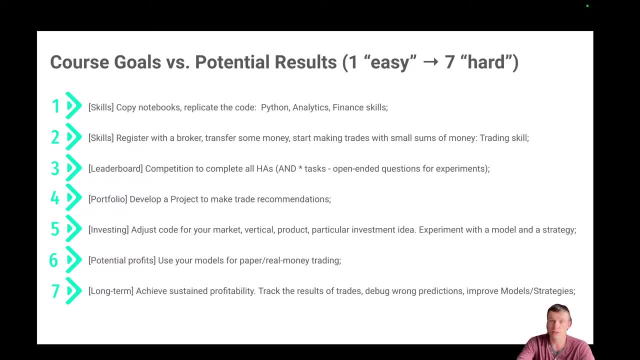 which I didn't mention during the course, something else which might be helpful for your market, for your project. Then, level number four, it's a portfolio. you can develop a project, you can create this project and that makes trading recommendations. and it is a good portfolio, addition to github. and if you ever try to work as a data scientist, analyst or just a software engineer, 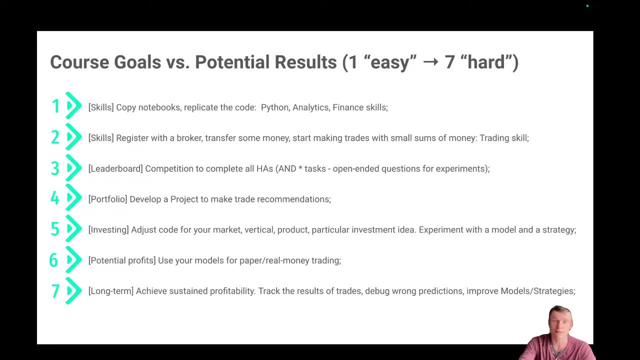 it's a very good thing to have Level number five investing. if, if you plan to actually use this course for investing, If you are investing already and after you build the trading system, you can adjust all the examples for your market, vertical product, particular investment idea. 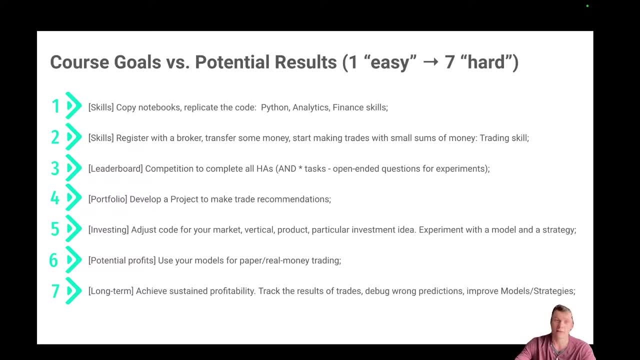 you can experiment with the model and strategy. Hopefully, if you do it for a long time, so you will get some profits. So this is a level number six. So it's it's not any idea, but it is a profitable idea. And level number seven: this is the. 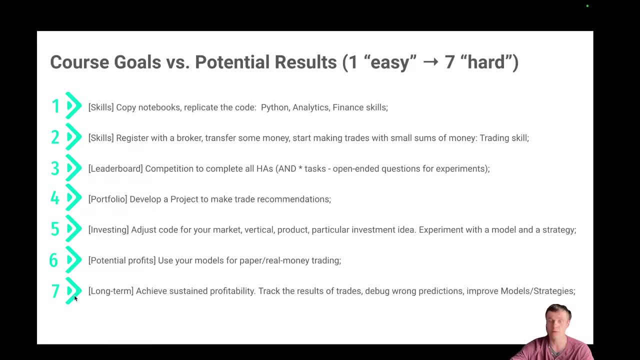 hardest and the ultimate goal, at least for me, that you can achieve a sustained profitability, that is, over the long period of time of 510- 20 years. you can. you can have a lot of trades using your algorithm And those trades on. 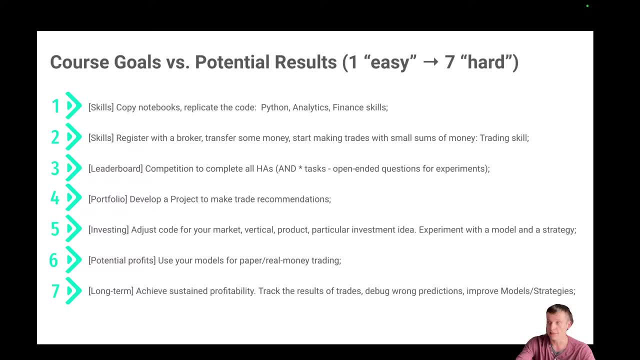 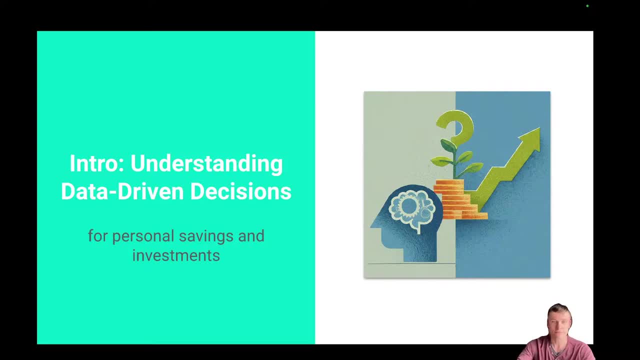 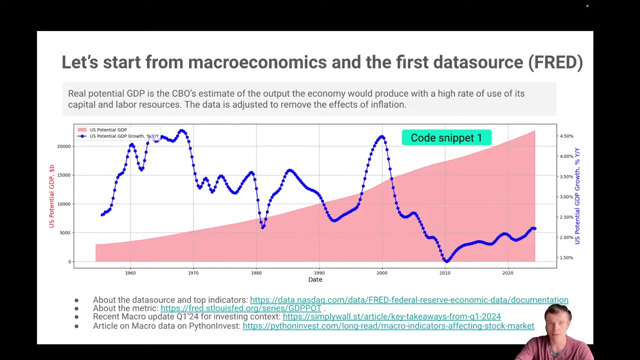 So let's move on to the next one. So let's move on to the next one. Let's start the introductory part. Why do we need to do all of this? And the easiest thing to start with is to understand the context. Of course, economic context is quite different in. 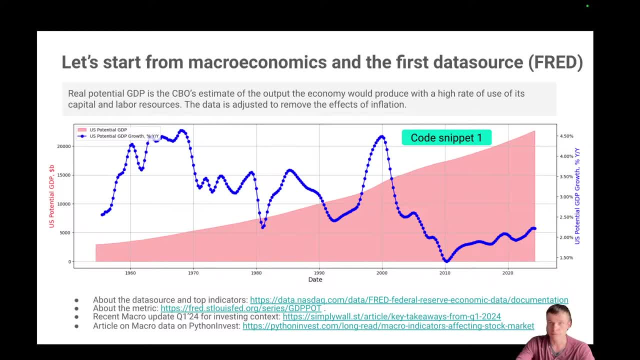 different regions and countries. So most of my examples will be about us or global markets. And for the US, You can start from the GDP. It is a well-known measure. It is a potential GDP in billions. This is a left scale and it grew for 60 years at some rate, and normally what we track is year-over-year growth. 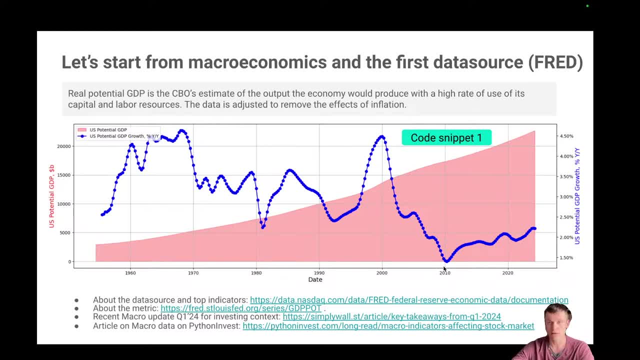 This is a right scale and you can see that from 2010 to the last year it is gradually improving and it is somewhere between 2% and 2.5% If you compare your investments or your income versus global economy growth. so over the long period of time it should grow, hopefully at least. 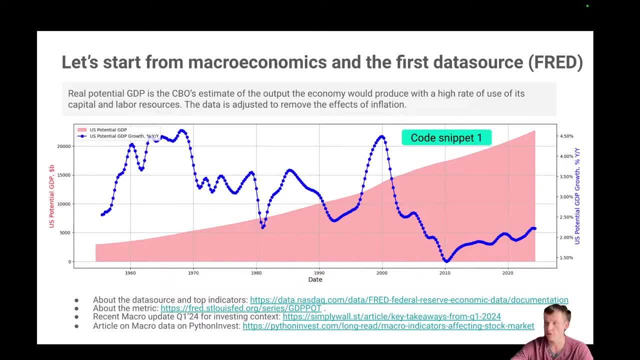 As fast as you see GDP growth in your country. You can read about this data series using this links thread. There are many other indicators on macro and articles. It's a good source to read. I also suggested you to follow some of the. 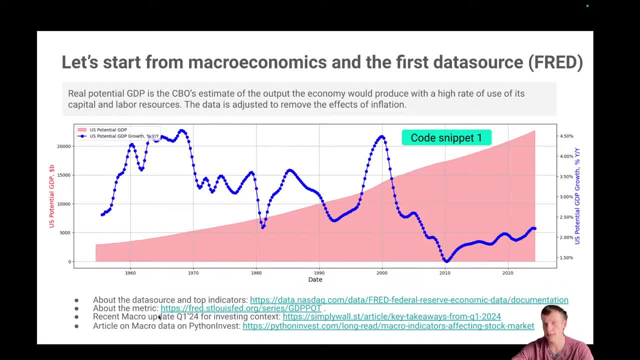 Data sources to get regular updates, and there was recently a macro update for Q124 from Simply Wall Street and they do have updates every single week, I believe, And some time ago I wrote an article about macro data on Python Invest. There are about 60 different indicators which I think are important and are connected. 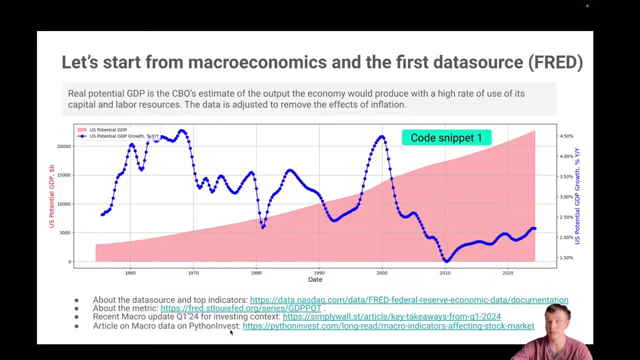 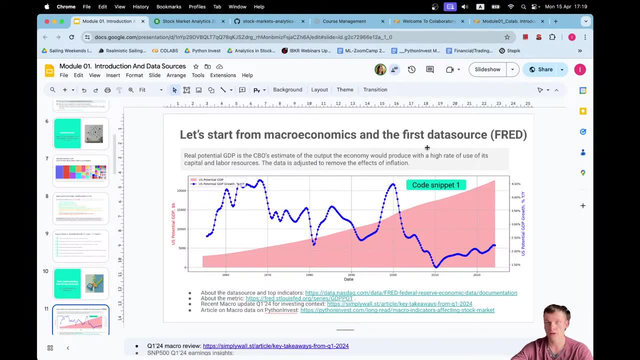 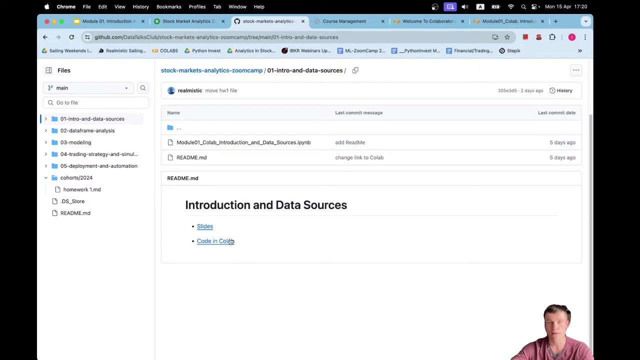 With trading activities in the US. I see there is a good snippet- number 1, so I will show you how you can get exactly the same data. You probably saw that we added slides and code on GitHub And if you click module 1.. 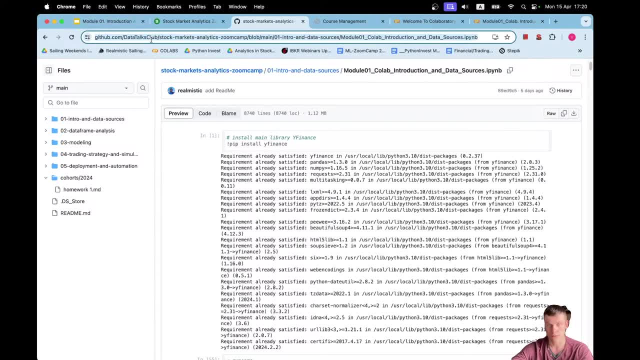 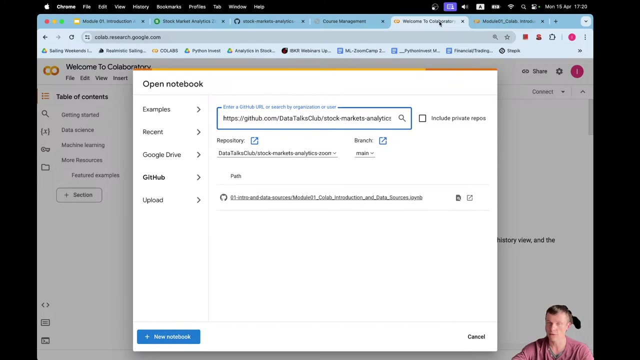 You have a the link for this notebook. I will show all examples that can be executed via Google Colab. Probably in most of the cases you can execute it locally, but it it may have some local dependencies and you may need to tune slightly the code. 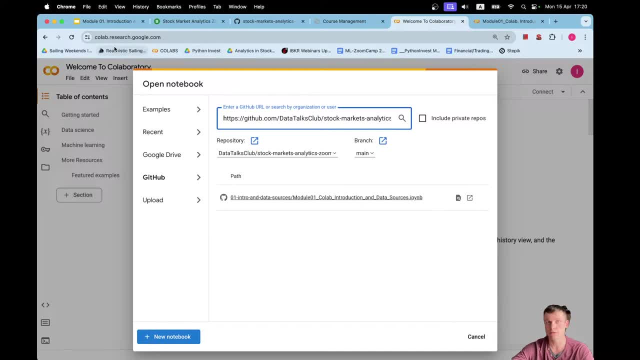 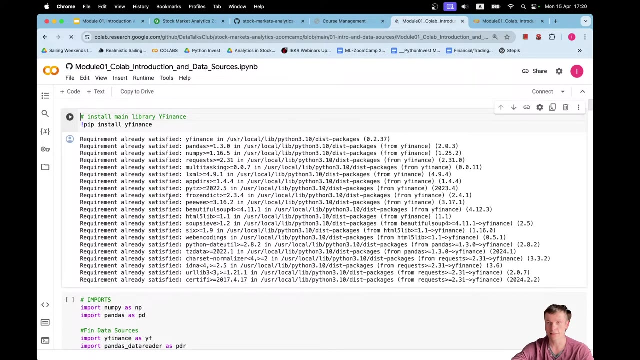 So if you never used Colab before, you need to open colabresearchgooglecom, click github, copy past this address. you will have it here, So I click it here. this is a new instance. this is a my local instance and I can connect, so 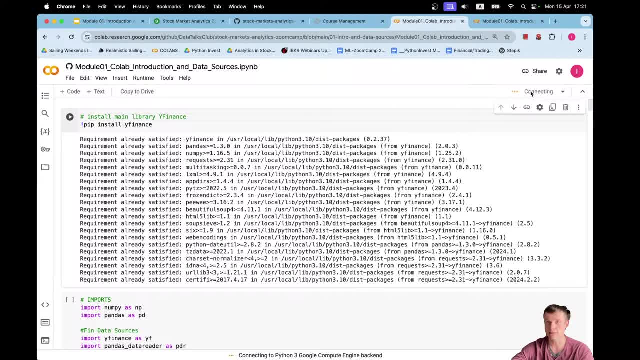 that's why it is a standard, standardized connectivity, standard libraries, and I try to write the code in such a way that you don't need to manage any dependencies. If there are some dependencies, like this module, yfinance- you will have it straight away that they need to be installed. And now I 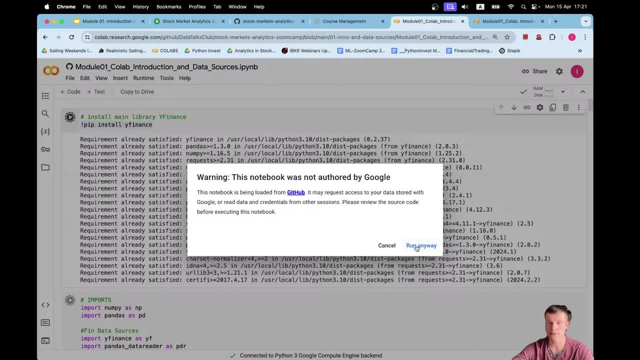 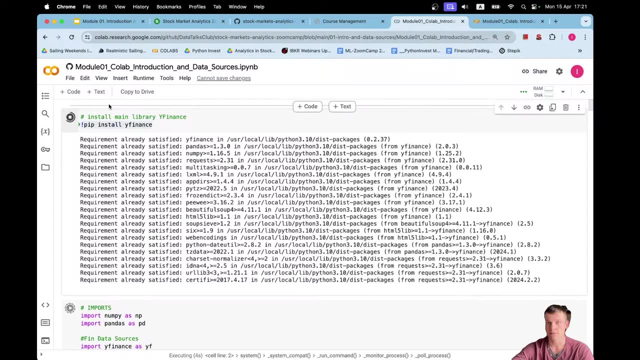 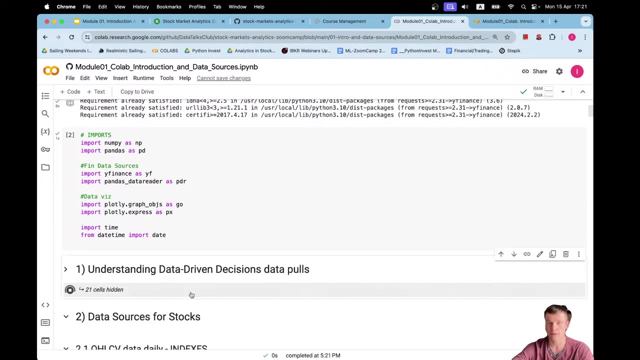 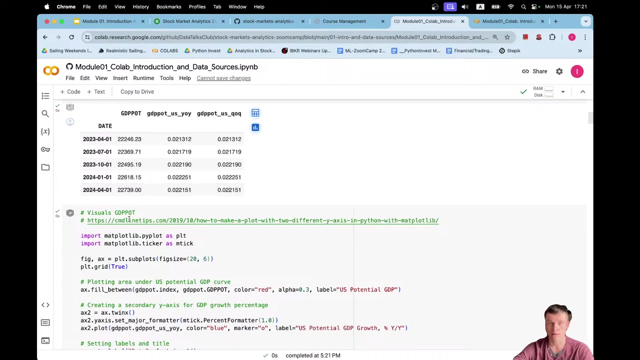 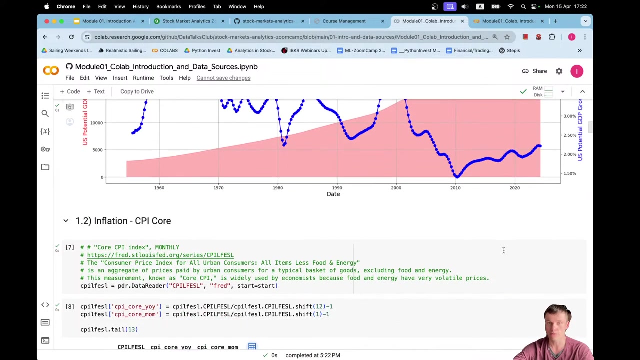 can run all. It says that it's a foreign Colab. I authorize it to run it and straight away I will receive the latest data and, as you can see, for example, last week there was no data for for the last GDP stats, for the last month or for the last CPI. 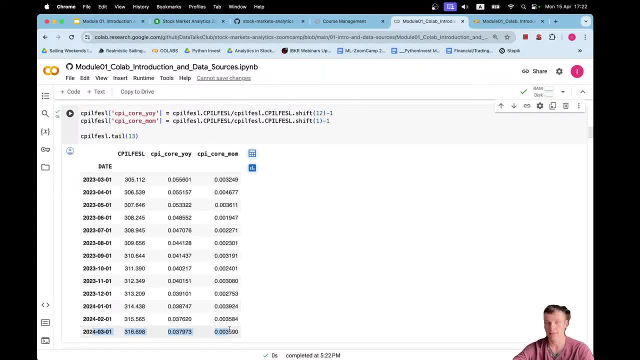 stats And today this data appeared and you can see that data. So this is easy, you can. 너 can see tthat data. So this is easy, you canhou. This is easy, you canou. this is easy, you canou. 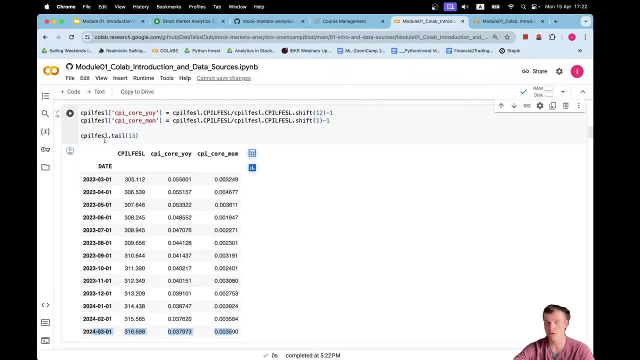 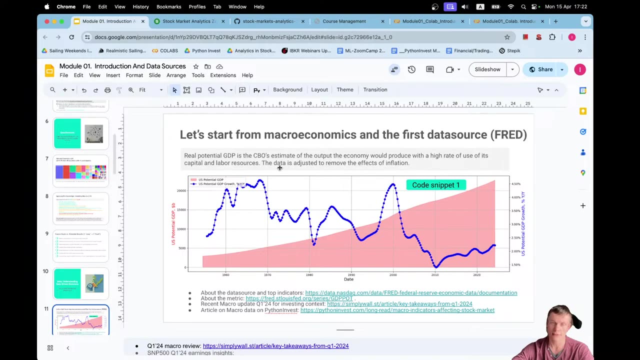 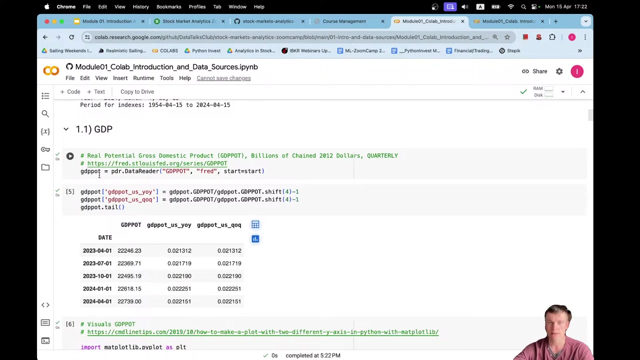 this is easy: you canou, you can run it, you can adjust. Now all objects are in the memory and you can change some parameters or some functions, And our first data set is US potential GDP. It is here, So, the only thing that you need to know, for. 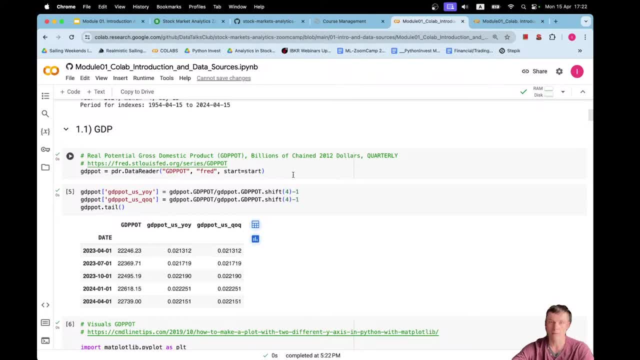 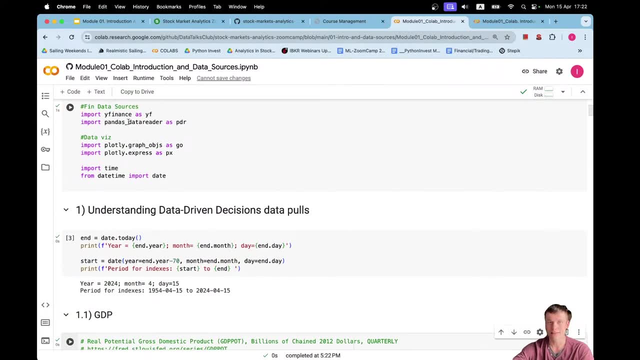 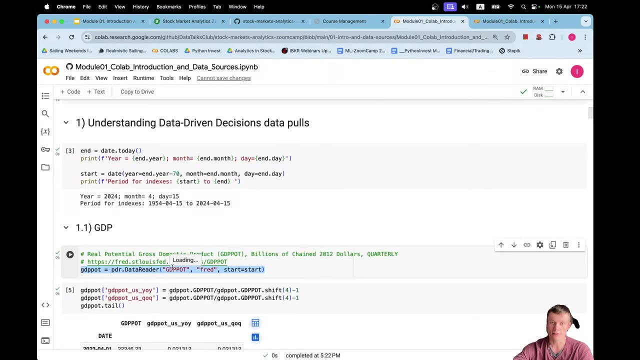 extracting data. for your homework is this line of code: You need to import pandas data reader as PDR and you need to write this pdrdatareader and show the time series that you want to download. You see GDP pod. It's exactly the same as you have it here in the URL address for 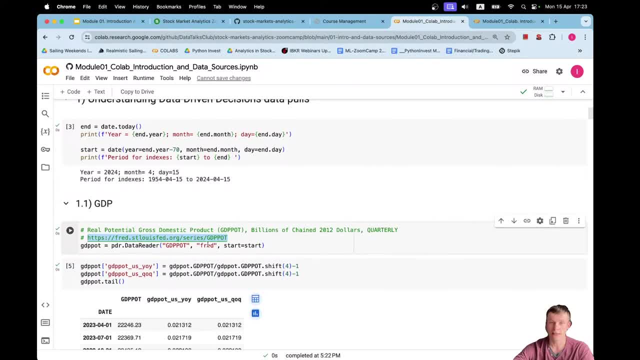 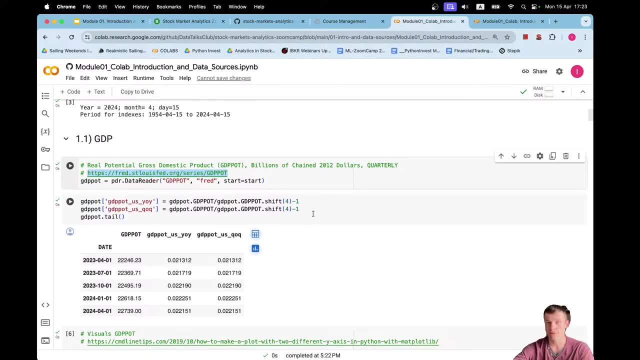 framework And then you will have a data. as a pandas data frame, I generate additional metrics that are year-over-year growth and quarter-over-quarter growth. I know that this data is quarterly. That's why I need to shift for four times a go to have a year-over-year 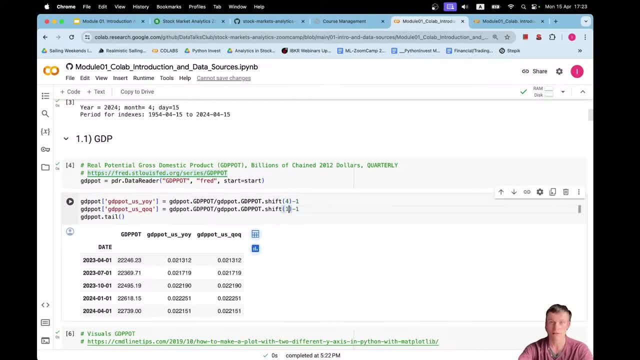 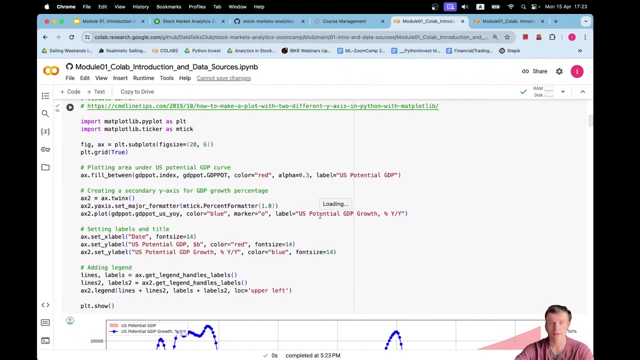 growth And here for quarter-over-quarter. here is a first error: that it should be shifted only one quarter ago. And then if you don't understand the details of this graph, that's not a problem. We don't use any complicated visualization, or you can. 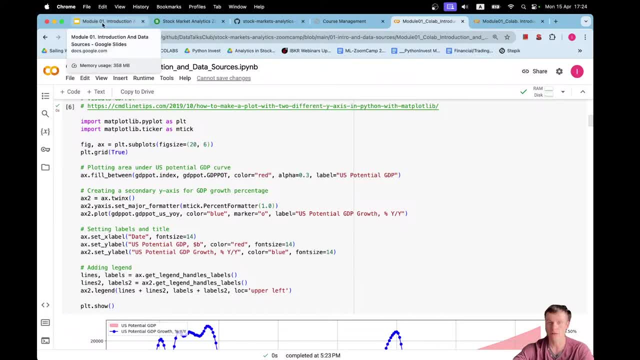 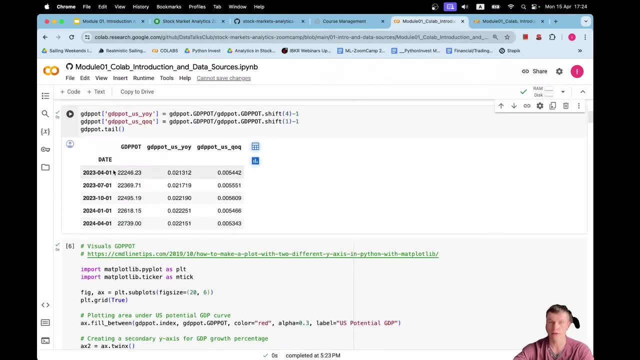 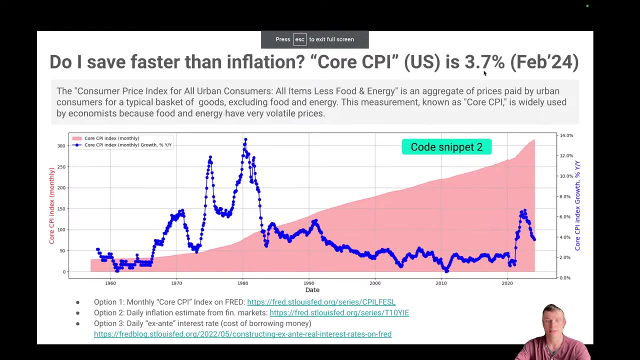 ask chat GPT to change or explain you the stats. The important thing is that you can download the data as a pandas data frame and you can work with the pandas data frame. Okay, let's move on. The second thing is core CPI or inflation. There are different ways. 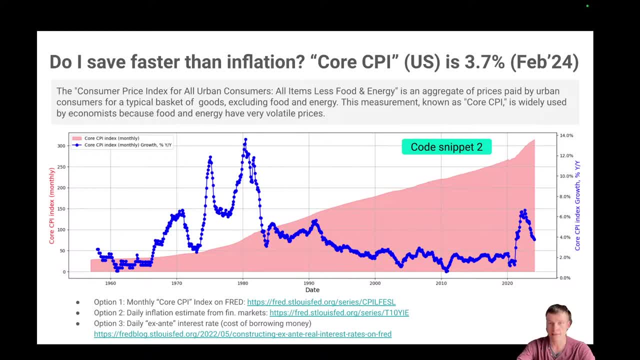 how inflation can be defined, And one of the ways which is commonly used is called core CPI And here, using exactly the same approach, downloading data from FRED using another time series data. So here you see: CPI, LFESL. So you need to know the. 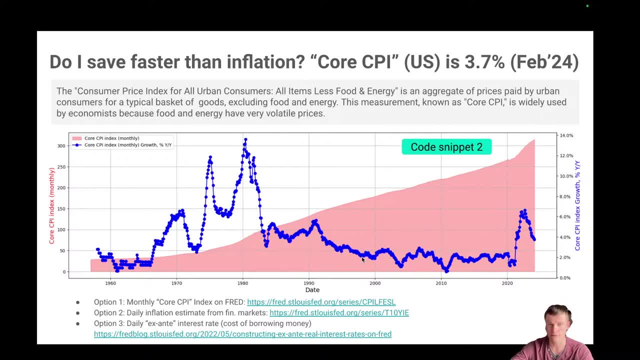 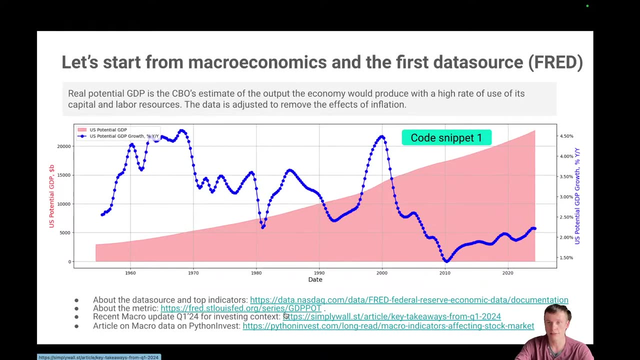 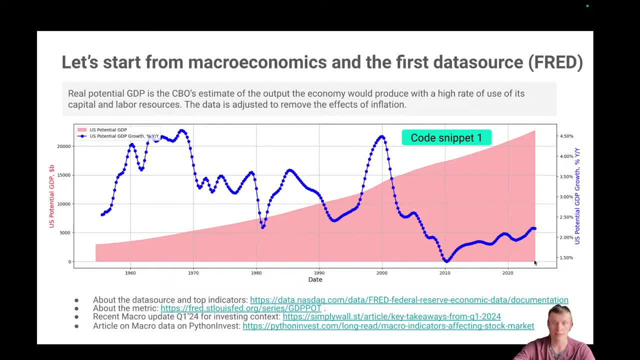 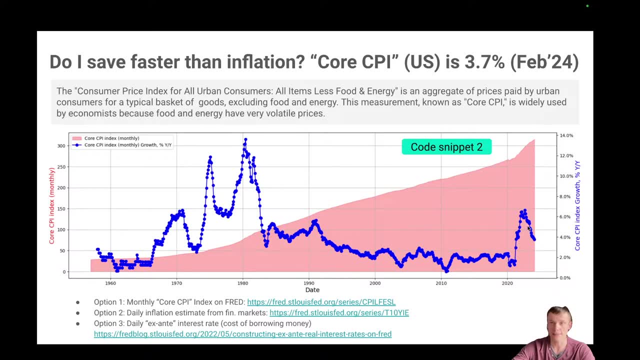 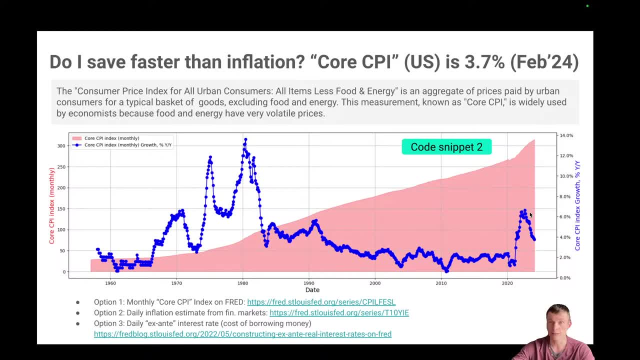 there was a spike to about 7 per cent in the US. in other countries, like UK and Ireland, the growth in the UK and Ireland it was about 10 per cent or even more, And now it's going down. So there is now again the growth in the US, as well as the FF2. 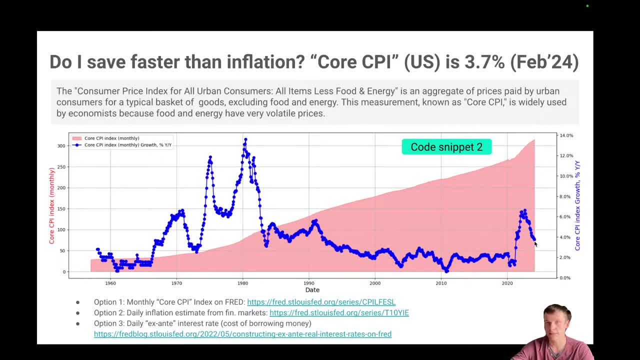 is some disbalance, but it is closer to you. as a retail investor or as a person living in that country, You feel that prices for products are growing up with the rate of inflation. There are many other ways to define inflation and you can look at the other parts of the. 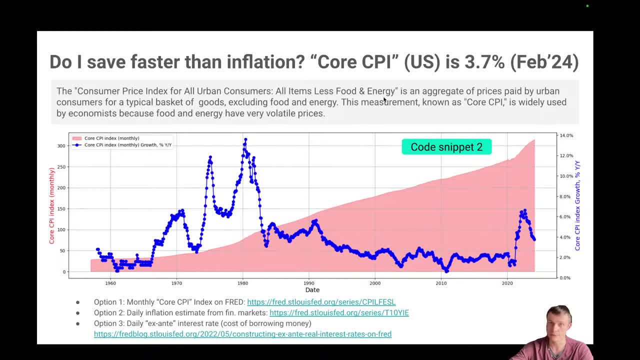 inflation. So this one does not include food and energy. You can look specifically at the food and energy inflation, especially if you try to analyze retail companies. Also, you can check the interest rates and inflation estimates on financial markets and those estimates- here there are the links you can read about them. There is an article. 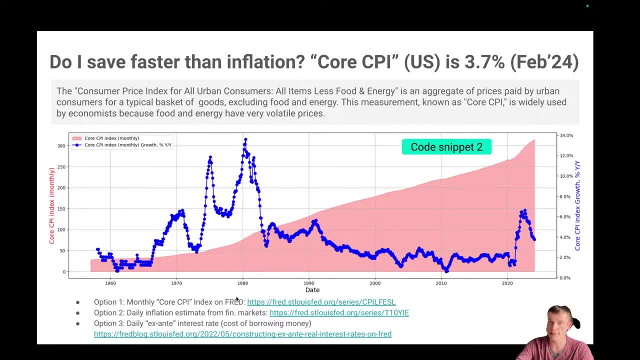 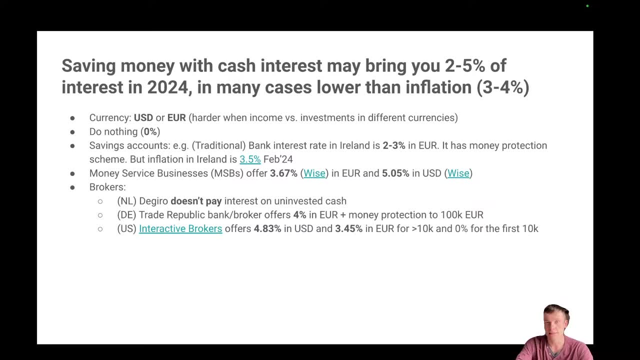 Thank you. These estimates are daily. they are not monthly and not quarterly. Now we have some economic context and if we start to save money just with cash, what can we get from easiest options that we have? Let's assume that currency is dollars or euro. 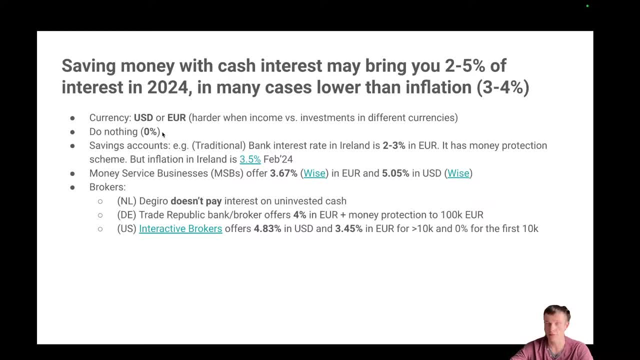 If you do nothing, you will get 0%. If you have your money and savings accounts- and many of them- they just don't pay any interest. This is not good because inflation is more than 0% and in 10 years you might lose like. 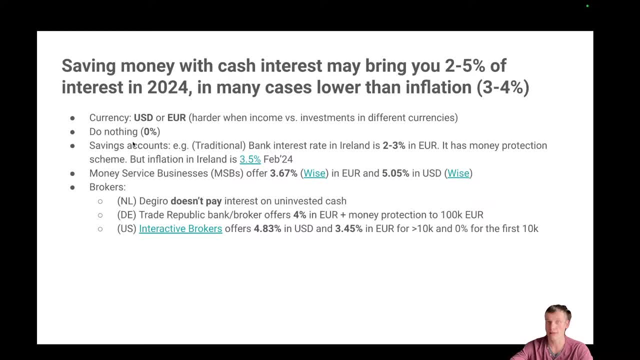 30% of your savings in terms of buying power, because you won't be able to buy the same amount of goods. So now let's think about traditional methods Like saving in a bank. In Ireland, you can get 2-3% of an interest rate in a traditional bank. 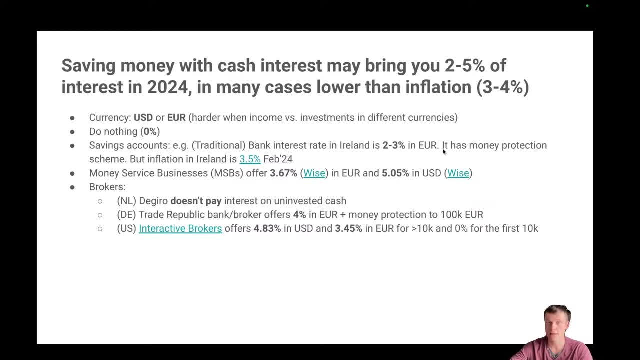 These savings are protected, usually up to some amount, But also inflation. in Ireland is about 3.5%, which is less than interest rate that you can get in a bank. Probably the next idea will be to go to the money service businesses like Wise in Europe. 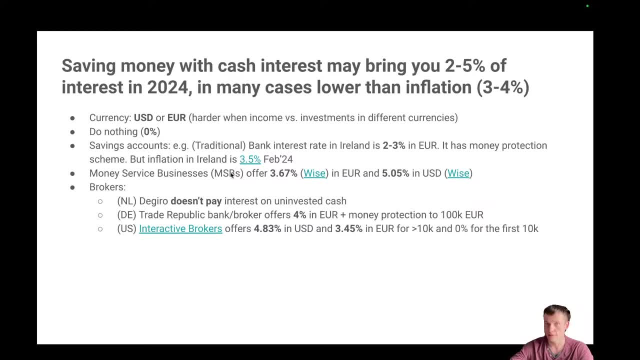 or other new companies like Revolut. They can offer higher rate of savings. Wise offers 3.67% in euro and 5% in euro, Which is not bad, But probably those money won't be protected by the government and by the money protected. 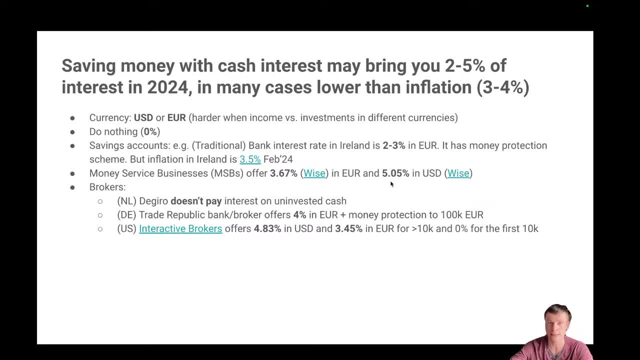 scheme Or they may be protected. You need to read the details. If you go to a broker- I used the Giro broker from Netherlands- they don't pay any interest on uninvested cash. If I use Trade Republic, a bank and a broker from Germany- it offers 4% in euro and money. 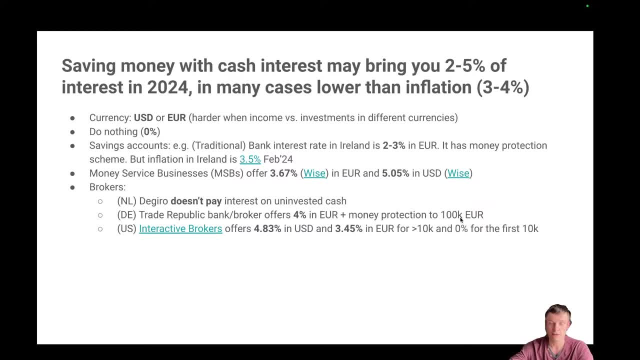 protection up to 100k euro. I never tried to use this, but probably it seems to be a good option to have benefits from a traditional bank and also to participate in investing. usually What I tried to use is Interactive Brokers. one of the biggest brokers in the US. 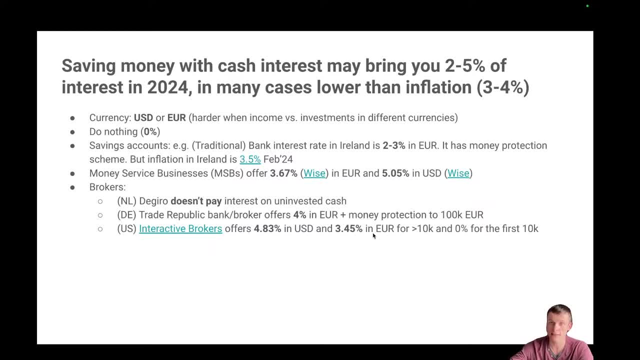 They offer 3.45% in dollars and 3.45% in euro, which is slightly higher than inflation rate that I have, But they also say that they have it only for money that are higher than first 10k of deposit that you might have. 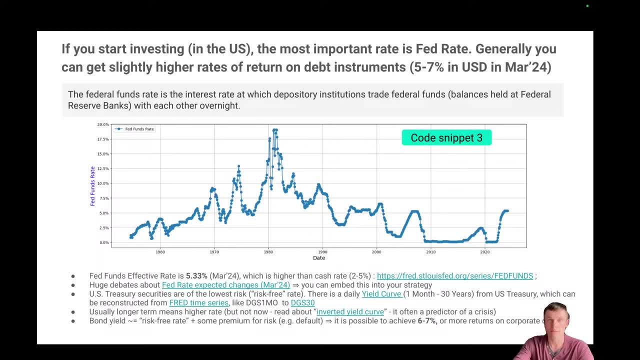 Moving to the next stage. If you start investing, you might want to compare versus Rates of return or versus cost of borrowing money, And probably the most famous and important rates, at least in the US, is a Fed funds rate. Federal funds rate is the interest rate at which depository institutions trade federal. 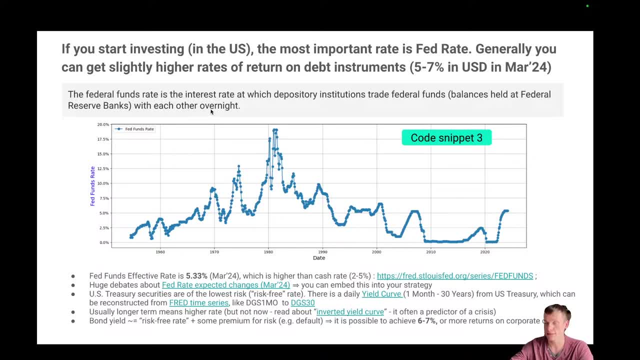 funds with each other overnight. Overnight is important. This is one day rate. This is a benchmark rate for many other rates. because federal funds is a government organization, It is treated to be not risky at all And many other rates, even if it's one day rate or overnight rate, will be higher because 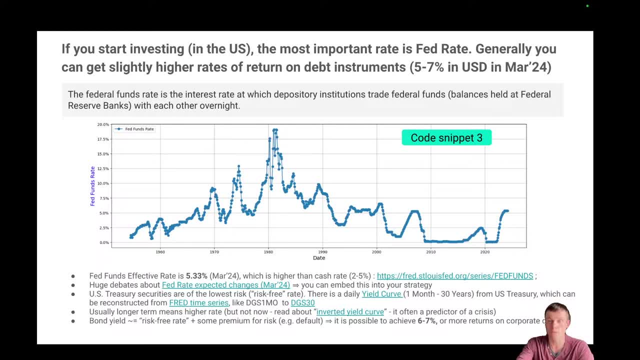 they have some risk that a borrower won't return money to you And normally If you lend money for a longer period of time- like one month, one year, 10 years- you should have a higher rate because someone who gives you money they might not have it back immediately. So they are locking those money and those money are not liquid and longer period of time. So it's it should be higher return, because otherwise they might do arbitrage and they might lend money for several shorter period of times and get a higher rate of return versus. 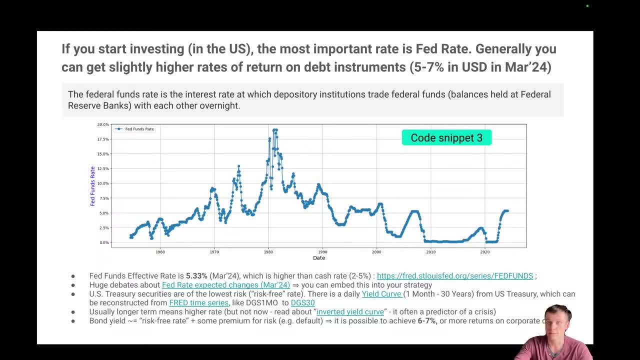 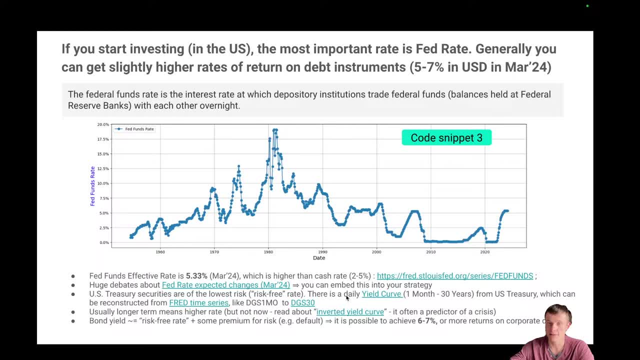 They won't lock money for the long period of time. Right now there is an interesting situation on the market that these rates are inverted for T-bills for a government's T-bills rate And there will be a home assignment for you to analyze when it was started. 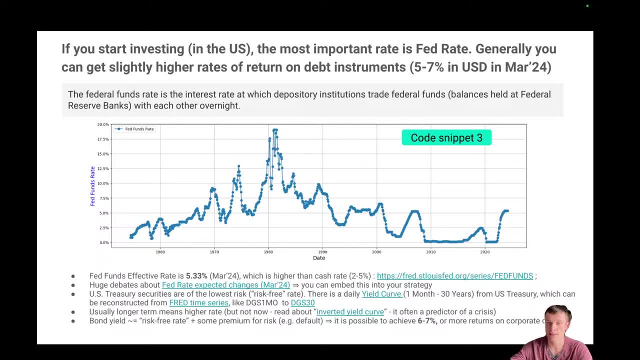 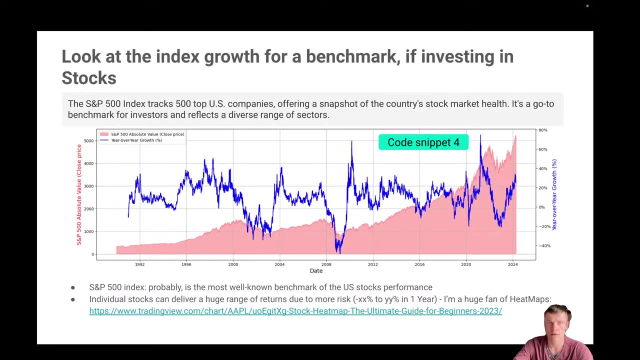 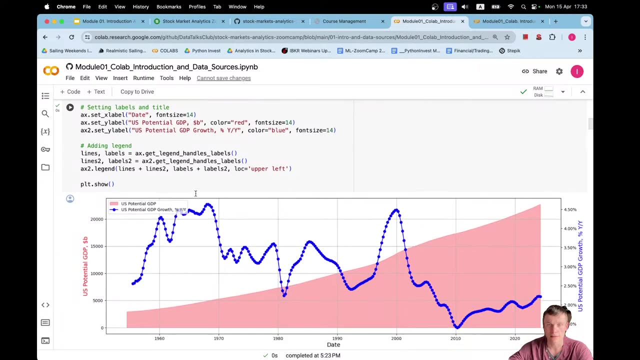 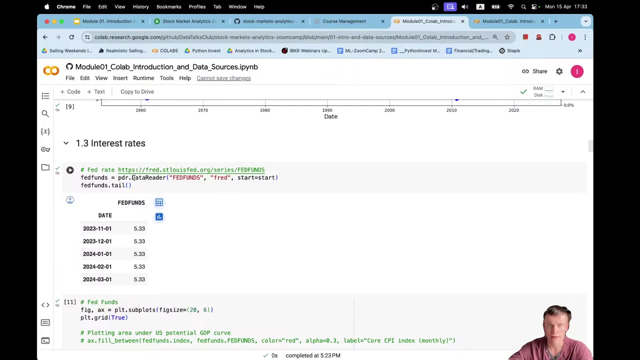 What's the biggest difference And so you can read whether it has any particular implications for a foreign investor. Okay, And got snippet number three. Let's look here. The algorithm is exactly the same. Fed funds: we use the same approach. 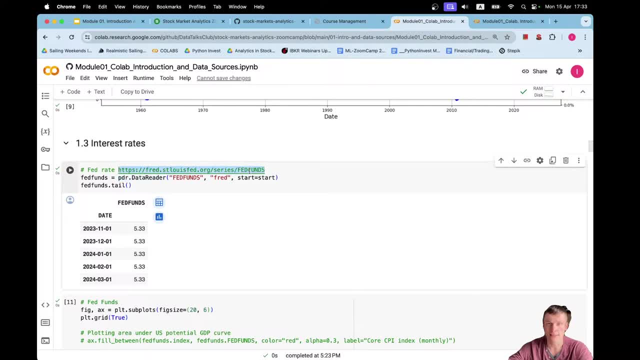 Here is an example. Okay, So we have a different URL address, a different time series. We call these methods, we receive an answer and that's what we have. This is a monthly Fed funds rate. It's exactly the same for the last few months. 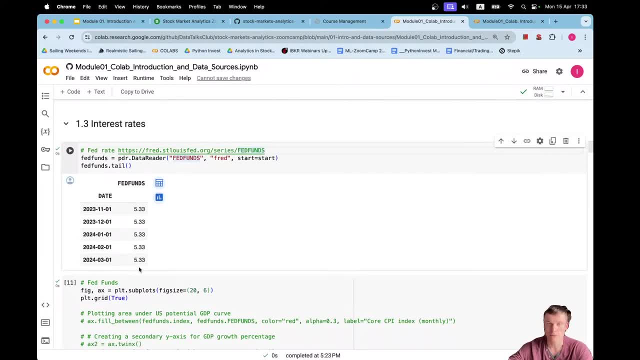 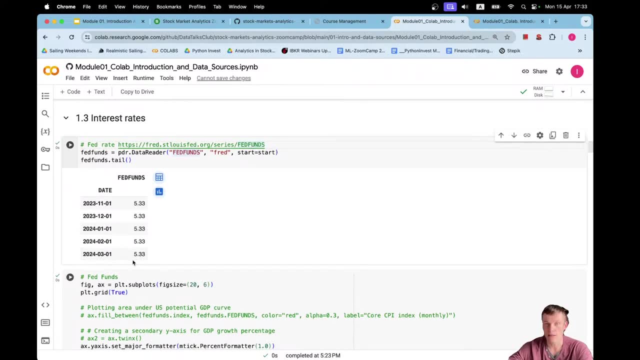 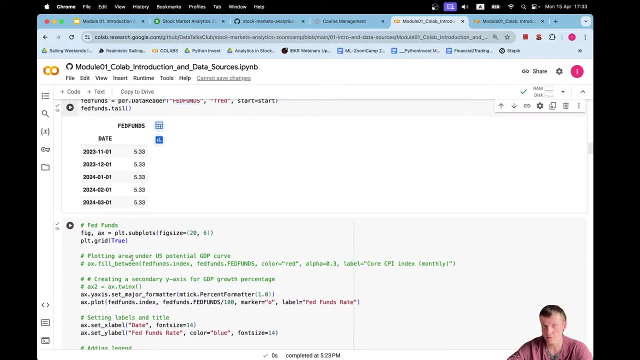 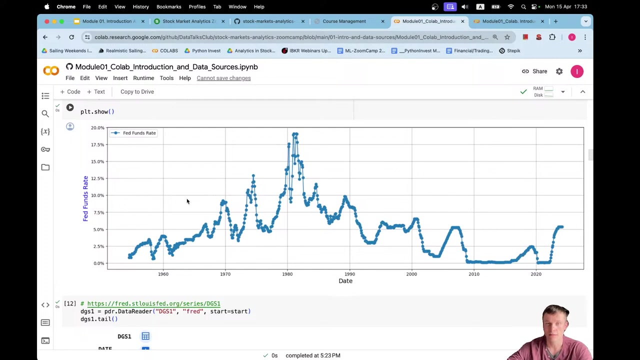 There are big debates and that's Fed will or won't reduce this rate And many market participants. They make predictions around this and make their own strategies around this. Visualization is slightly different. We don't have any relative metrics. We don't need to calculate growth rates. 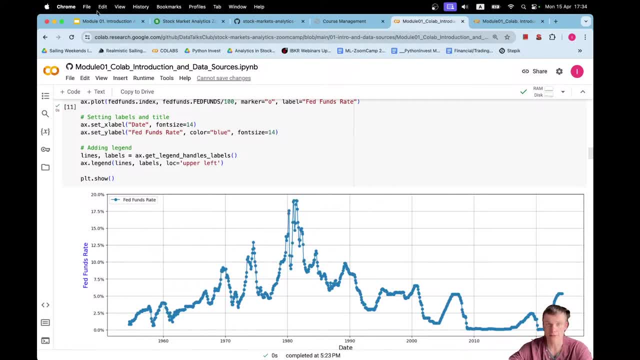 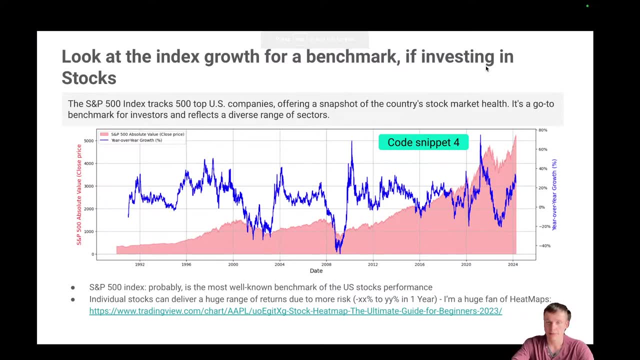 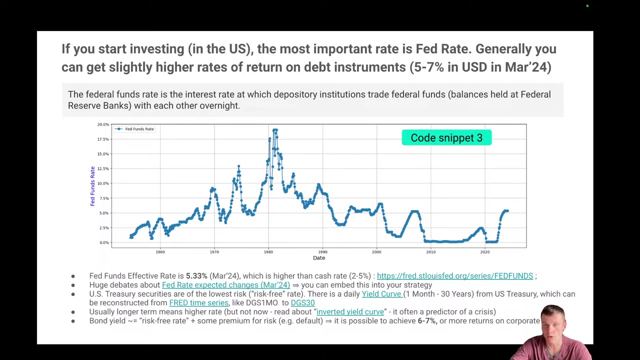 And here we have only one line time series. Okay, What do we have next? Next step. So if you understand approximately the rates of borrowing money, so for Fed funds it is 5%, For corporate bond markets it's probably 6-7% in the US. 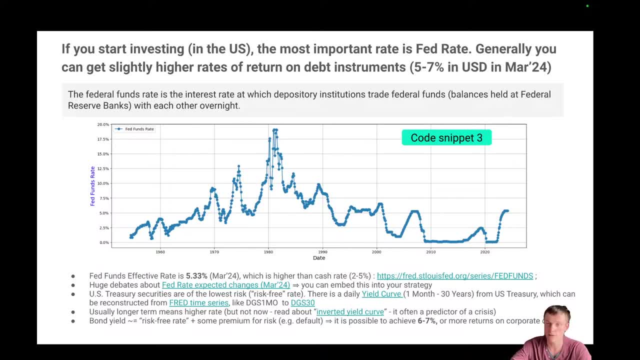 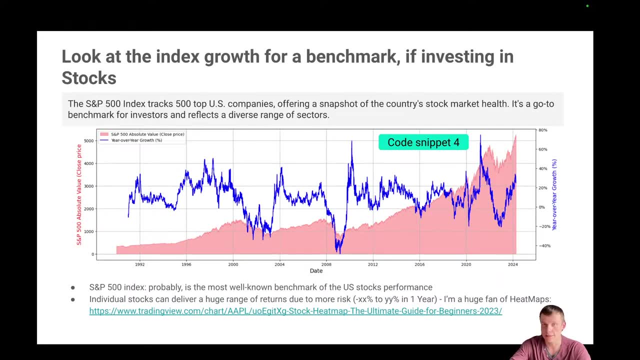 It is higher than what you can get in savings accounts or in GDP growth, but still. Next thing is to look at the stocks markets. Okay, And the most well-known benchmark for the US stock markets is S&P 500, and that's what. 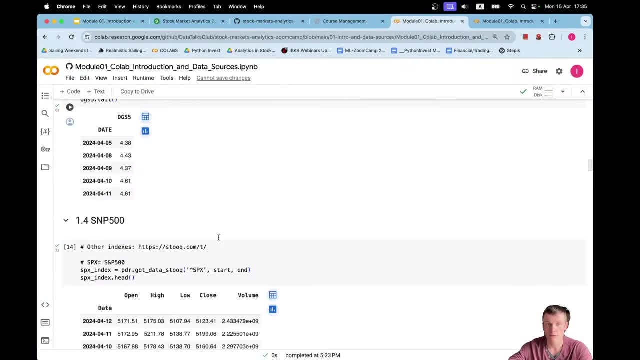 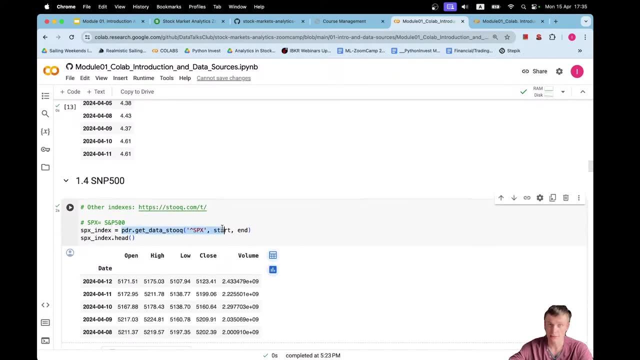 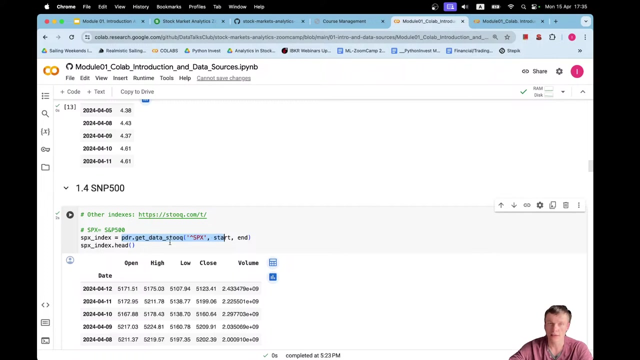 we exactly did in this section. We have S&P 500.. Here I have a different data source stookcom. So Pandas data reader. They implemented. They implemented different functions and different ways of accessing the data And you can get it from Yahoo Finance, which we will discuss later, or from data gets data stook. 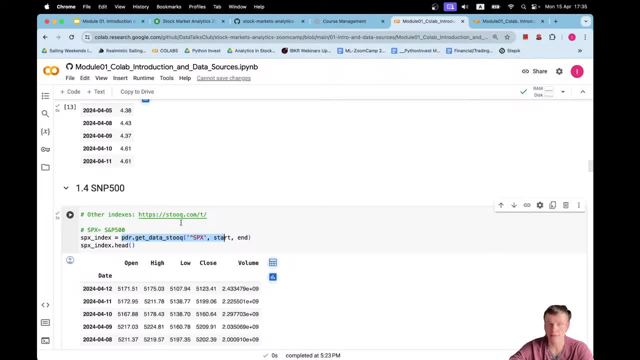 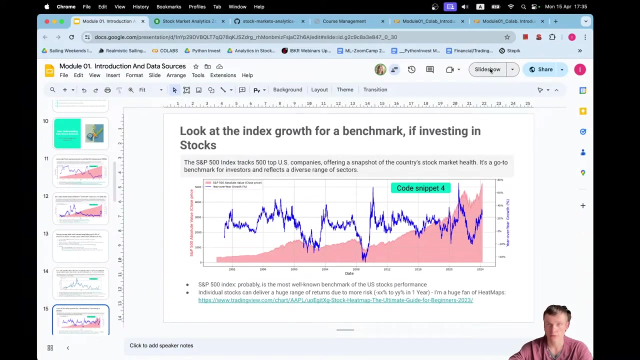 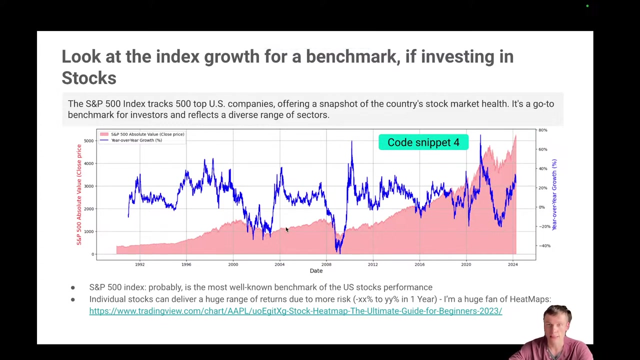 And on stookcom there is a number of indexes which you can obtain using exactly the same methods, but probably looking at the Indian stock market or Mexican stock market. You will just need to substitute this ticker and you will get the data. So for S&P 500, the situation is as following: 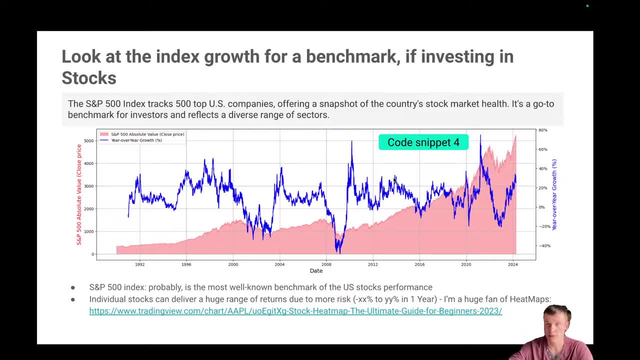 It is growing very often, but not always, And specifically in the last probably two years or so, it has been growing very fast. So it is growing more than 0% And lastly, it is about 20% year over year growth. 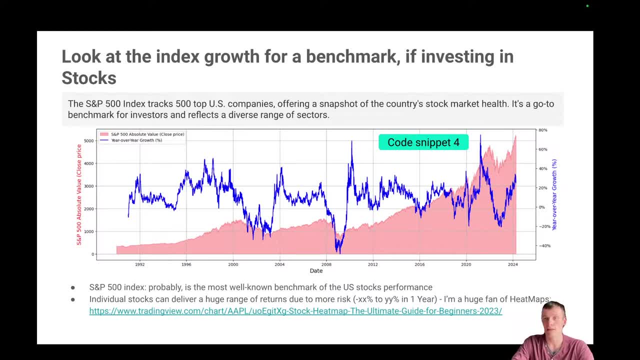 That means that you might want to be involved in the stocks trading. The problem with that is that sometimes it can go down 20% or 40%, So you might not want to invest all of your money Into these type of assets. But you can guess that sometimes these type of assets- stocks or stock indexes or stock ETFs- 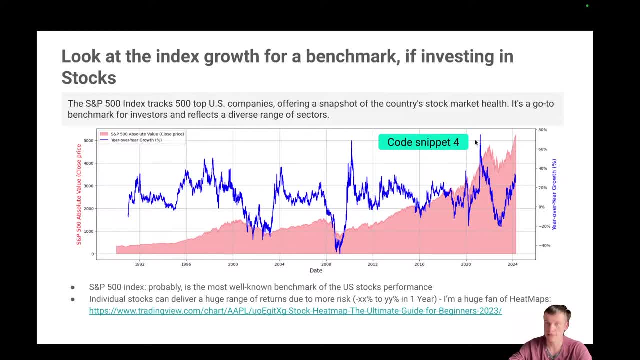 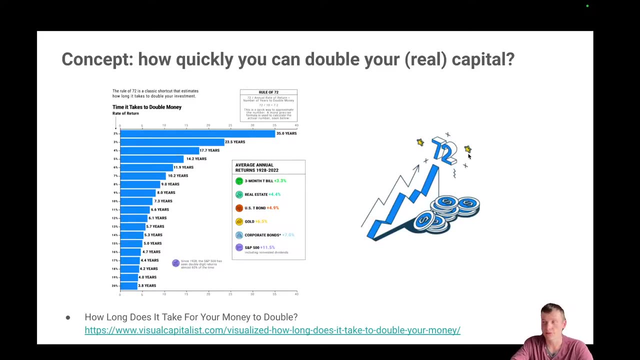 it can have a very high growth rate, And your benchmark can be exactly this index or some mix of indexes, And your benchmark can be exactly this index or some mix of indexes And you will track against this benchmark. And now let's think about real implications of investing into different types of assets. 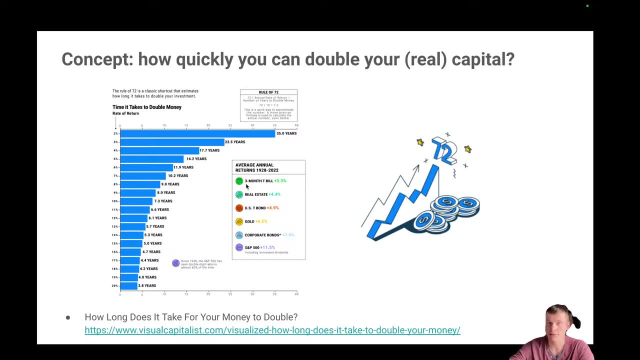 For example, if you invest in three months T-bill, there are ETF funds and you can get this rate. The average rate of return is about 3.3%. The average return is probably 5%. Five years ago it could be 2% or 1%. 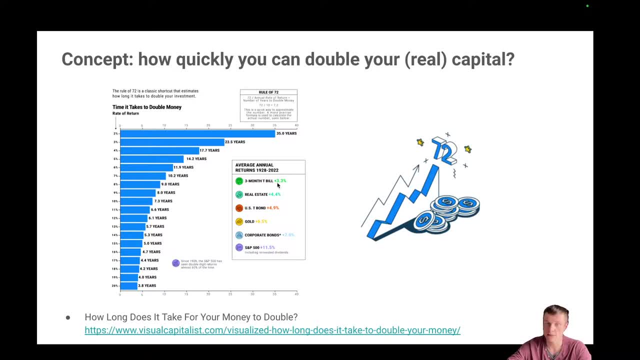 But normally it is more than zero, It is just very small. And then if you go into real estate, average return is 4.4% In T-bond, is 4.9% In gold, 6.5% In corporate bonds, 7%. 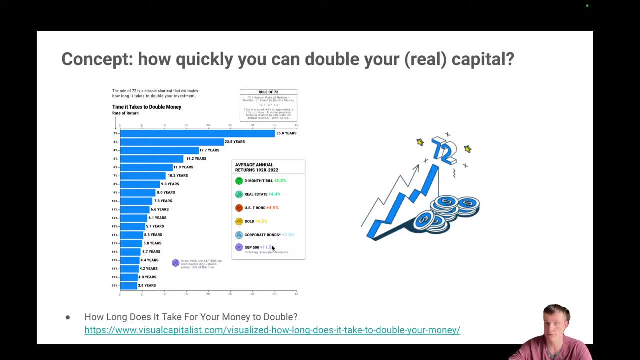 And in S&P 500, 11.5%. The difference is that if you receive Just a 3% return on your investments, it will take you 24 years to double your capital, And if you go into S&P 500, it will be six years. 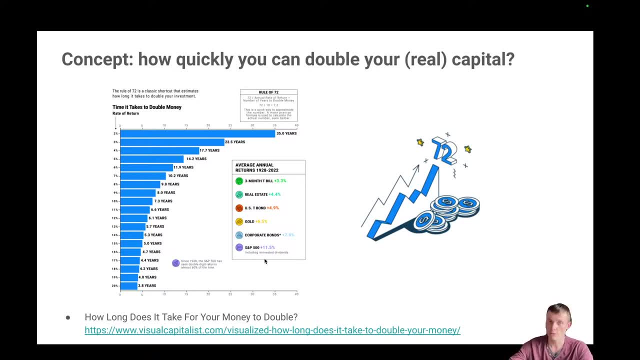 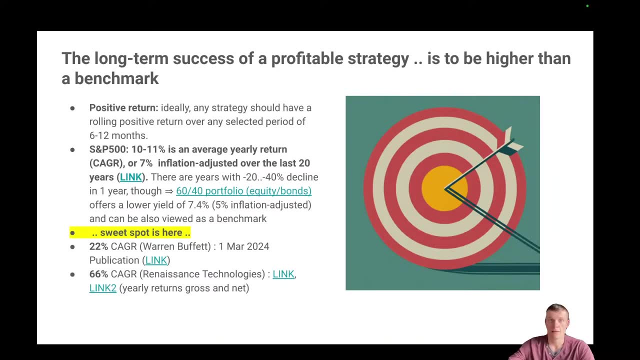 It's a four times difference, But it's not always like this. It is an average growth over a big period of time. Now let's combine everything that we have Here in the introduction if you want to develop a profitable trading strategy. first thing, 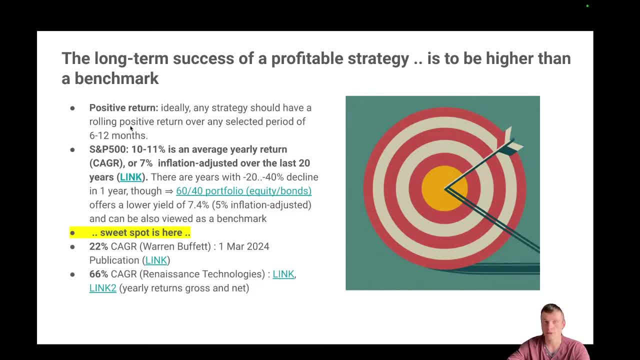 we want that any strategy should be positive in returns And in the local momentum. in one day, in one week it may be negative, But if you take rolling returns over the last one month or six months you should try to make it. 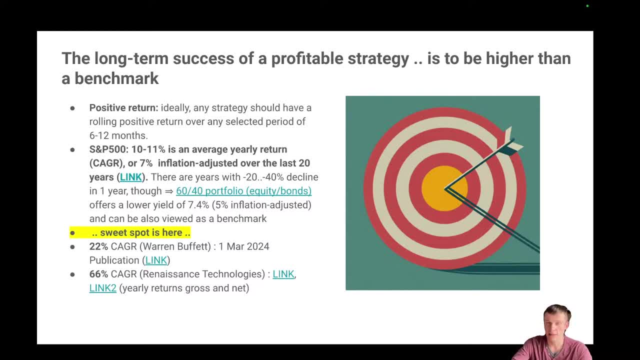 At least positive every given period. If it's not positive, probably you need to shut down the strategy for a moment, You need to update it, You need to start another strategy, And so on. So then we saw that S&P 500 is 11% of an average yearly return. Or if you subtract inflation, it is about 7% of the return. Often times, S&P 500 is 10% of the return, But if you subtract inflation, it is about 7% of the return. Sometimes, as I said, the people consider a mix of S&P 500 or stock markets and bond. 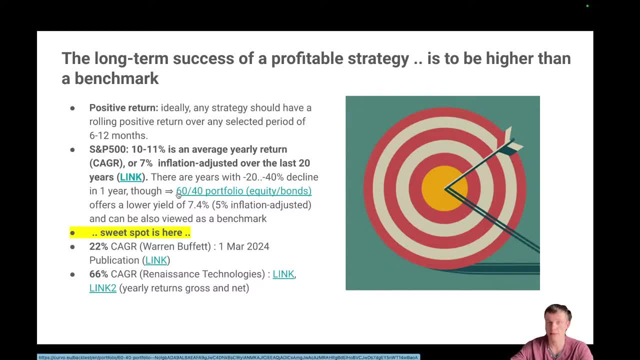 markets. This is called 60-40,, 60% equity, 40% bonds, And that means that you sacrifice some of their long-term returns. You might have a smaller yield or smaller return of 7.4% or 5% inflation. 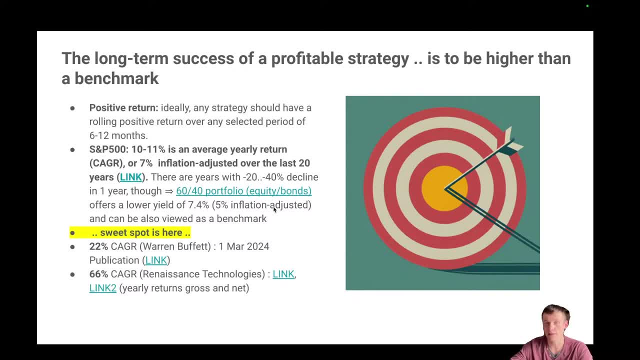 Right And you can use it as a benchmark to compare for your future strategy. You just need to decide what trader you are, what's your risk profile and what's your period of investment, And now it's a sweet spot here. So everything that grows higher than everything before it's already a great thing to have. 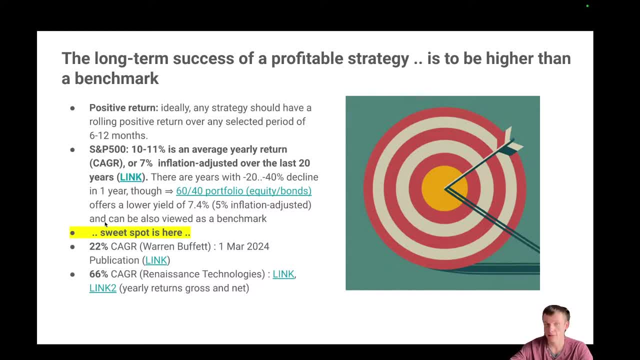 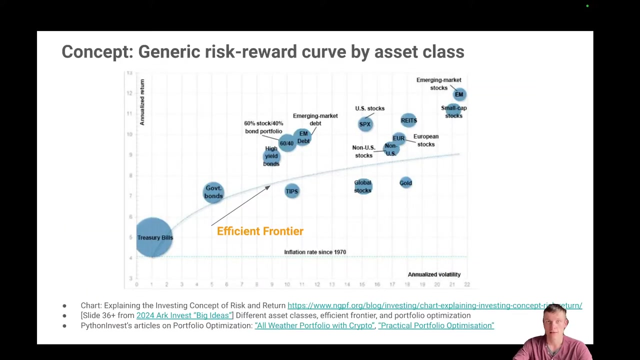 So that's it, Thank you, Bye, Bye, Bye, Bye, classes. as you saw, in previous slides, we we discussed treasury bills returns. we discussed 60, 40 stock bonds, portfolio US stocks and there may be other types of assets which you want to combine somehow and if you combine them in specific. 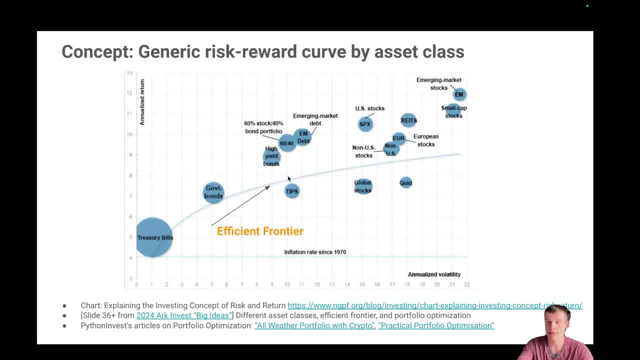 weights. you might have characteristics of your portfolio which are good for you. for example, you want to optimize with overall return and you don't care that sometimes your portfolio can be down for 30 or 40 percent. or you just don't allow your portfolio to be down for more than 10 percent and you want to optimize in. 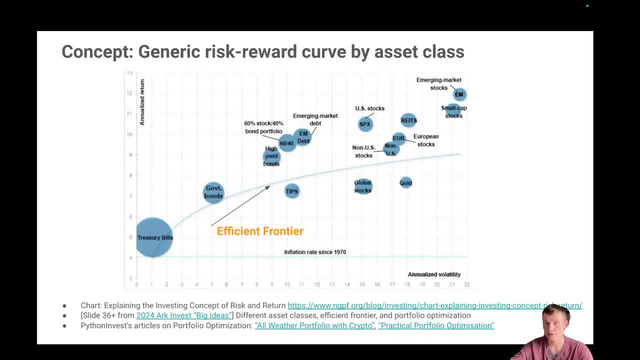 such a way that your drawdown is not bigger than 10 percent at any given time. that's why economists they developed this efficient frontier line and it actually says a simple idea: that's, if you want to achieve some combination of achieve the best performance from some combination of assets, you need to combine them in a 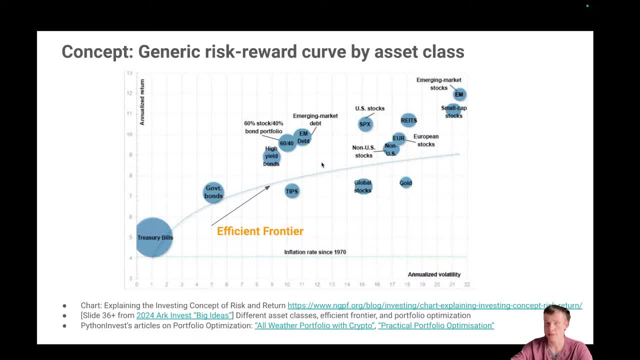 special way and you will have this efficient Frontier line and the the shape of this line says that when, when you try to achieve a higher analyzed return, you will have, you will generally and generally have a higher volatility or higher risk. so that's, that's the trade-off, that's if, if, 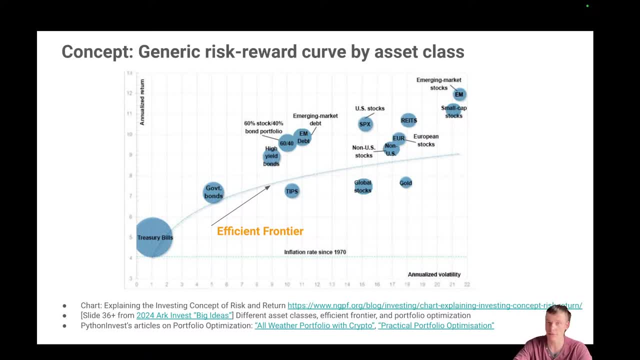 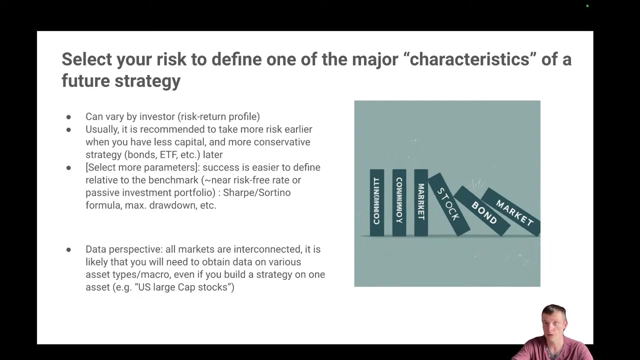 you want to to risk more and bad for for higher yield yields, you will have bigger fluctuations. I wrote articles about this over the portfolio with crypto and practical portfolio optimization, and the code is there. please, please, read um. now let's think about your, your project and future characteristics of a trading strategy that 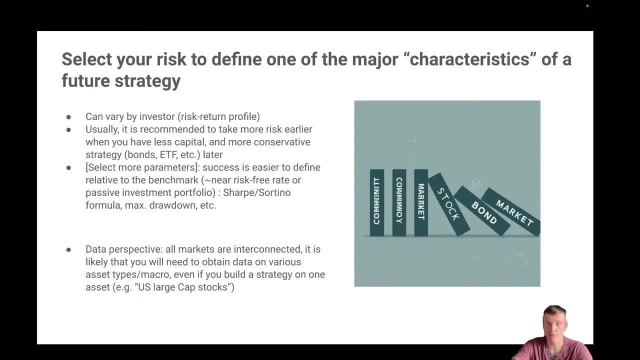 you might want to develop as as your capstone project. the first risk or risk return profile can be very different by investor and you need to decide what. what is your risk, that that you you wanna bet, and then usually what I see from from the literature, that if, if you are a young investor, you don't have a lot of capital, it's it's recommended to try. 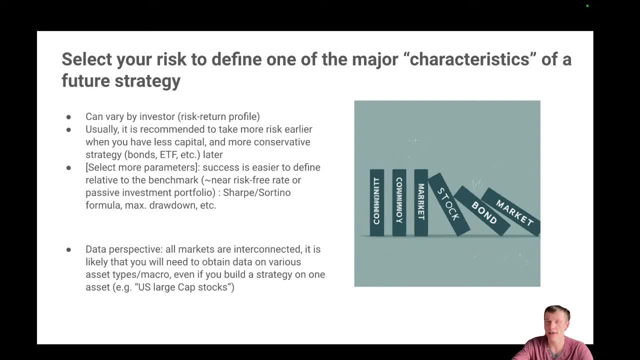 different strategies and to to have slightly more risk and then when um when you have some experience and when you have a higher capital uh, you take a more conservative strategy. um next. um next is to select the, the Benchmark to uh to trade against. um. probably the easiest Benchmark uh is a 6040 portfolio, or just SNP 500 portfolio, if Kalai. 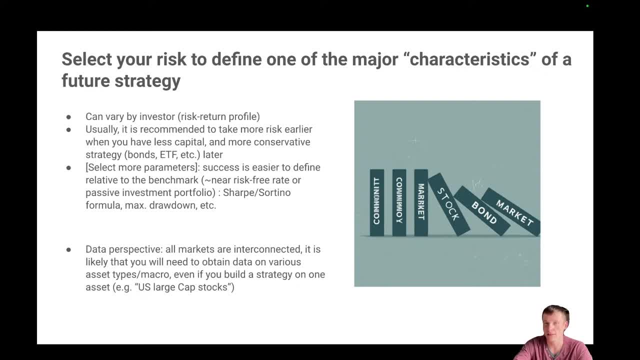 if you are investing in the US, If it's other markets, just select a benchmark for the index in that market and you will have that benchmark. The idea is that sometimes the overall index goes down and it is natural that your strategy may go down as well. but if you go down less than, 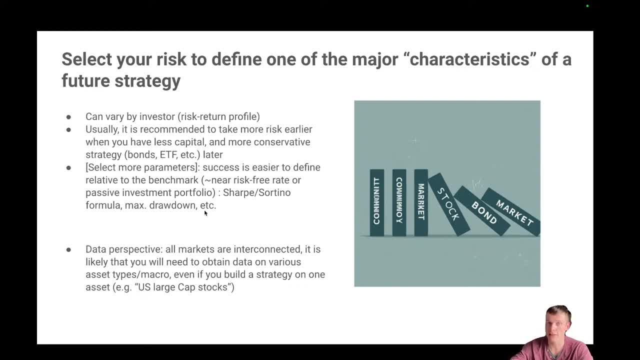 the benchmark. that means that your strategy is working and you are generally better off than a generic benchmark From the data perspective. the thing is that all markets are interconnected and you need to check this. You need to download different macro indicators, other asset types like. 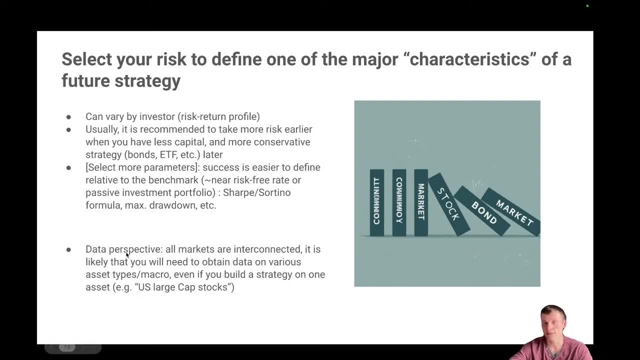 gold commodities, bonds markets, equity markets, global, local and check correlations and try to model. So you need to read about the strategy of the market that you want to invest in and think about what metrics, what features you will need to participate in building a good strategy. 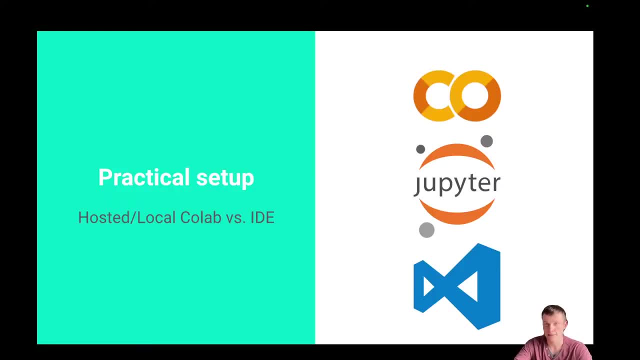 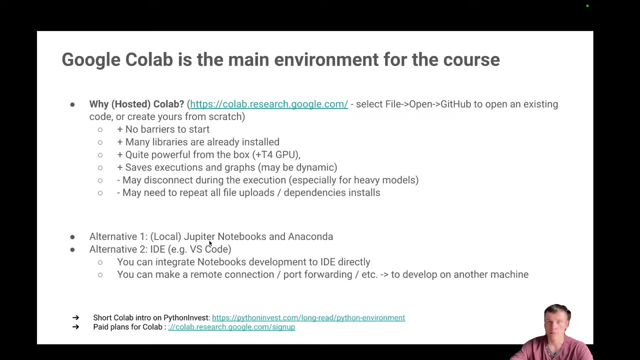 So now let's move to the practical setup. I already showed you how to work with Collab, and my first article actually on the Python Invest website was about Python environment, and you can read this article following this link: pythoninvestcom- slash- long read slash- Python environment. So why do we use Colab? First, it's 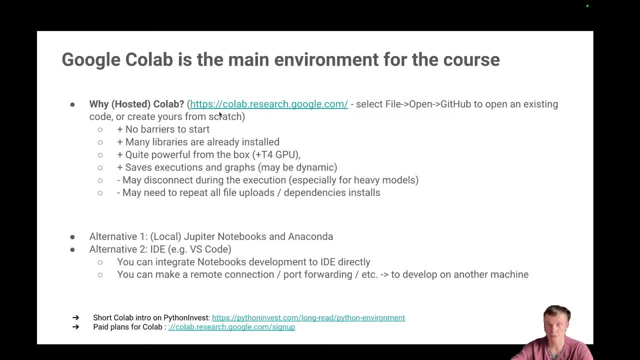 very easy. You can reuse my code. you can share your codes on GitHub and other people might use it as well. There are no barriers to start, or small barriers to start. Many libraries are already installed on the machine. It can be quite powerful from the box. Actually, you can have T4 GPU for free. It's not. 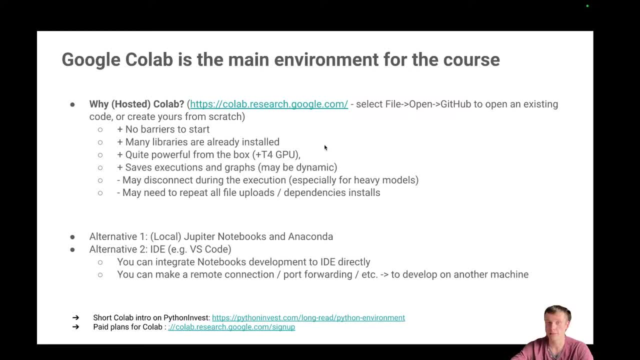 guaranteed time, but you can run a deep learning model and it has some power. What I really enjoy to have as an analyst is that all executions are saved and you have the results of them stored in in a notebook, and some of the saved executions, like plotly express visualizations. 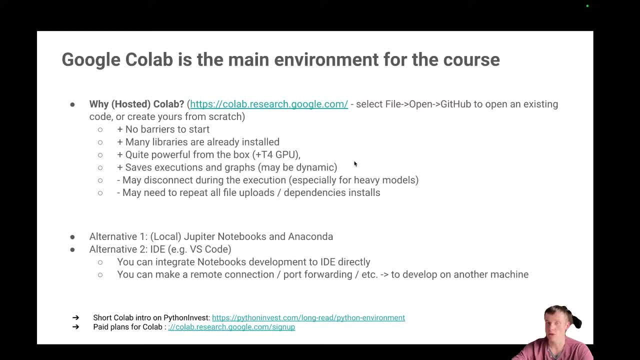 they might be dynamic, so that you can access them even after visualization, and you can have much more than you can get from a just a static table. the pros of this approach is that it's not guaranteed that it will execute for for a long period of time, especially if you 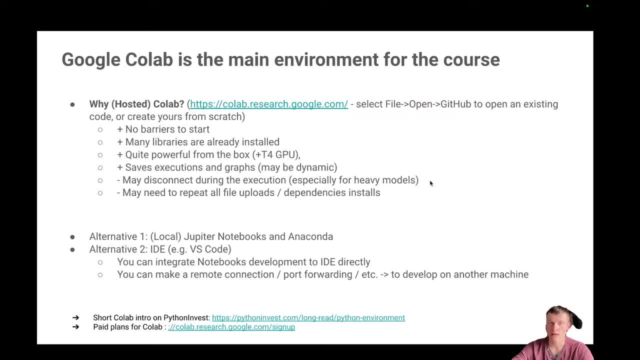 have some heavy models. you may need to upload anything that you want to use as a file, or you need to save it on a google drive or somewhere else and write the code that can access it, and there are several alternatives. for example, you can use local jupiter notebooks on anaconda, or you can use ide like vs code and you can even integrate. 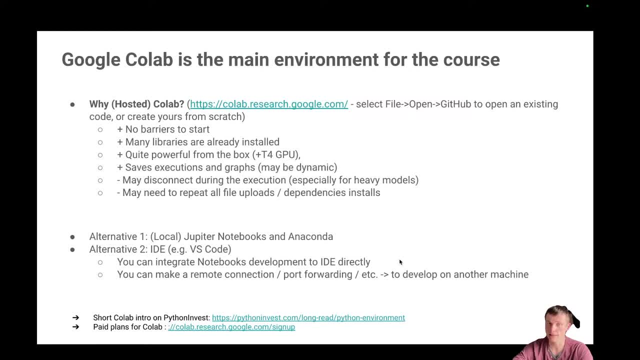 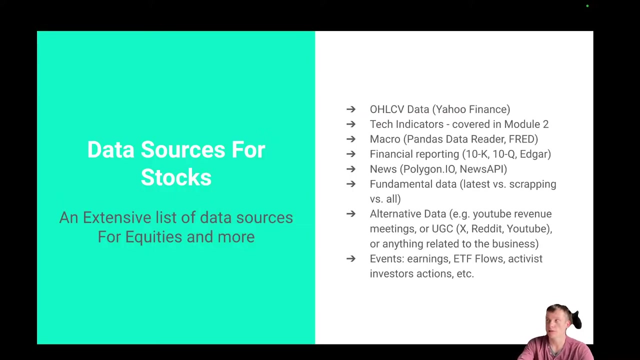 notebooks to develop in this id, or you can make a remote connection, port forward in and develop on another machine. we won't need this until the last moment, the last module of automation. everything before that we will do in in colab. so now let's talk more deeply about data sources for, for stocks and many of them. 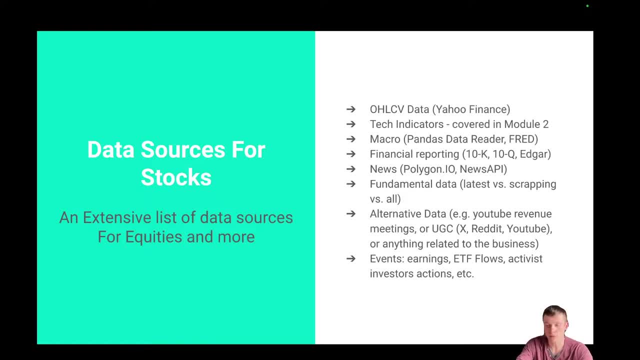 can can be used for other financial assets as well. so our first data source is yahoo finance, which provides daily or minute or hourly data on open, high, low, close and volume data for many, many different types of assets. one natural idea on on these data is to generate tech, technical indicators. it will be. 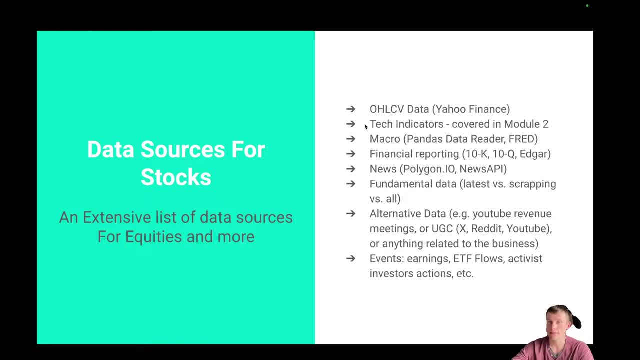 covered in module 2 because it's a technical way of working with with the data and producing additional features for your stock market, and you can see that the data is being generated by these for your data frame. I've just wrote an article about it. hopefully I can record. 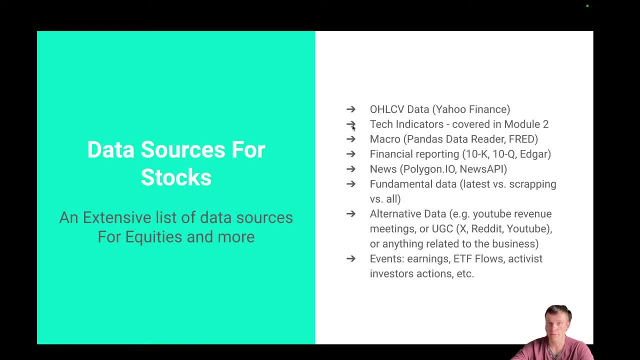 a video on it in in one week. and then we discussed briefly macro data source, which is Fred's in in my case for 90% of the macro data and I use pandas data reader library financial reporting for US stock markets. it's Edgar, I have a. 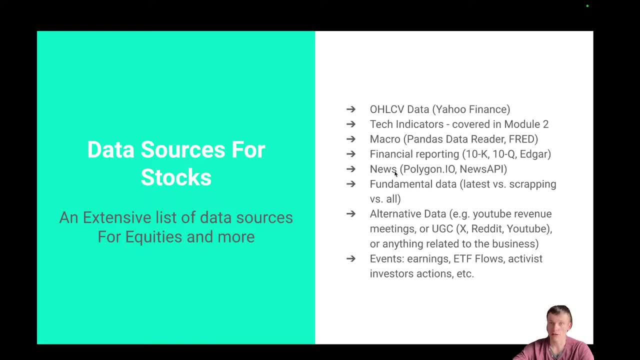 slide about it on as well. for news I used two news providers. it's polygonio, it's actually paid financial data with the free tier, and it has a lot of different endpoints, not just news. but it was quite convenient for me and it was quite convenient for me, and it was quite convenient for me and it was. 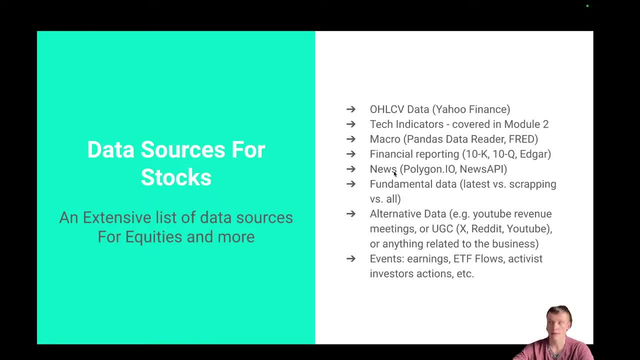 enough to use it as a at the free tier. but before that I wrote an article using use API and at that time, about two years ago, it had a longer period of freely available history, which is quite good thing to have. then fundamental data- normally it's it's available easily for the few latest periods, for example, if 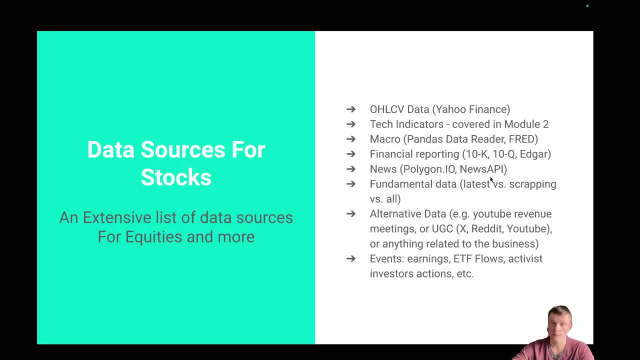 you go to the Yahoo Finance, you will be able to get it, but not always. if you want to use 10 or 20 years of history for fundamental data, you will need to pay for this or do web scraping. there are many other data sources like alternative data. it can be. 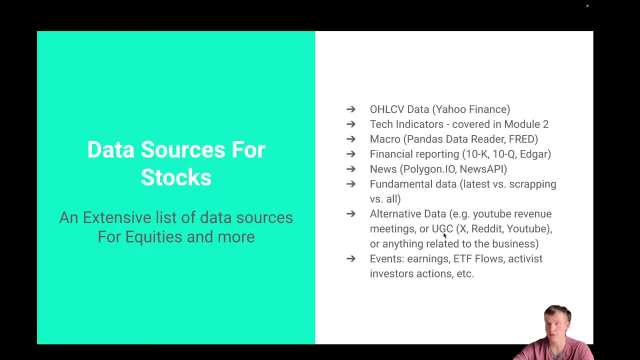 YouTube revenue meetings, user generated content, Twitter or X, Reddit, YouTube or anything else related to the business. we will discuss later the examples of this data. and also one additional type of alternative data: it's events data. probably you, you want to design a strategy around some events. for example, it is well known that during the earnings season- and it's 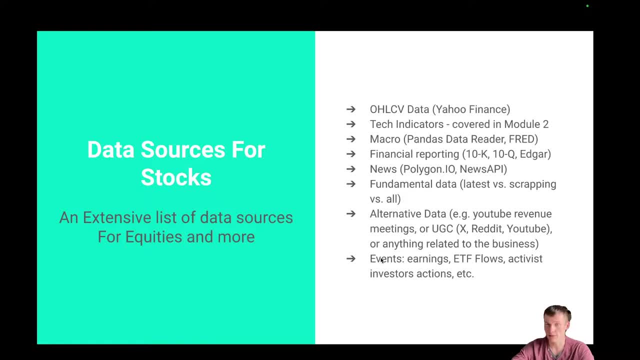 just started for for the q1. in the US more and more companies they are just reporting earnings in in April and during earnings season. if the reporting is is good, there are- or bad. there there are- stock price fluctuations, so you might want to catch this and you might want to look for some interesting data. 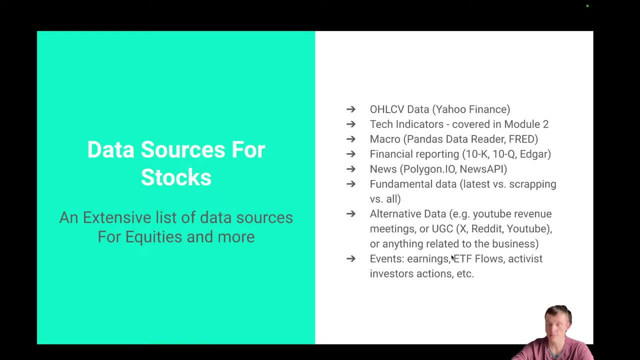 might want to know in advance what are the earning dates. Another example is ETF flows. Exchange-traded funds are the biggest participants of the market. They are institutional investors and if those ETF companies decide to invest in this or that stock, it may change the price of a stock considerably. The 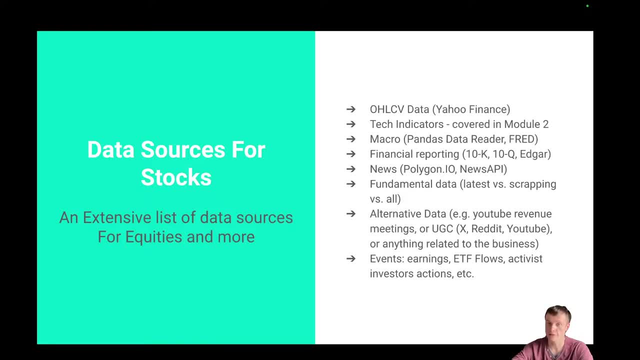 problem for us is that they report on their investments only quarterly and only with some lags, so you can't see it in real time. Probably it's hard to design a strategy around it, but still you may be able to do something. Activist investors actions. There are specific type of companies who 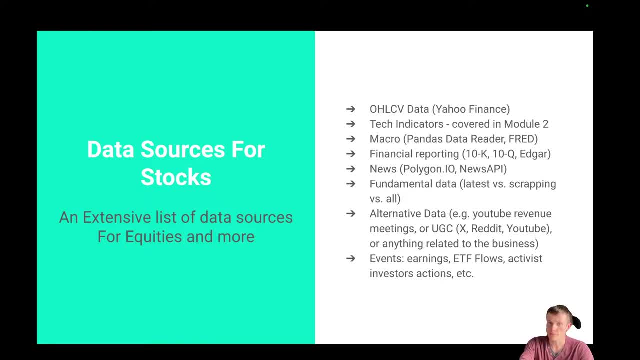 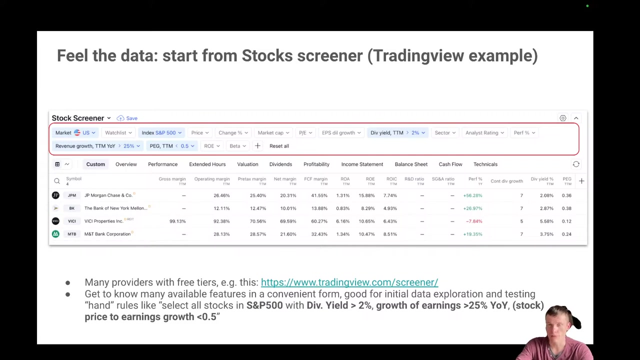 participate in activist activities and you can read articles about it. you can follow these companies, you can check their reportings and probably design a strategy around this as well. So let's check in detail all these data sources Before we go in coding. I would suggest you to look at some stock screeners' tools. I 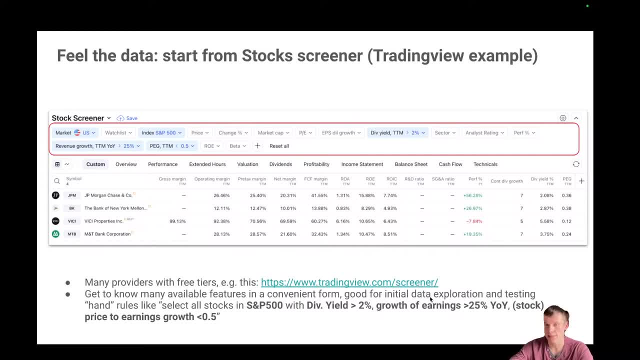 would suggest you to look at some stock screeners' tools. I would suggest you to look at some stock screeners' tools. I I personally like TradingView slash screener, but there are many of their contents available, Just for you to understand. 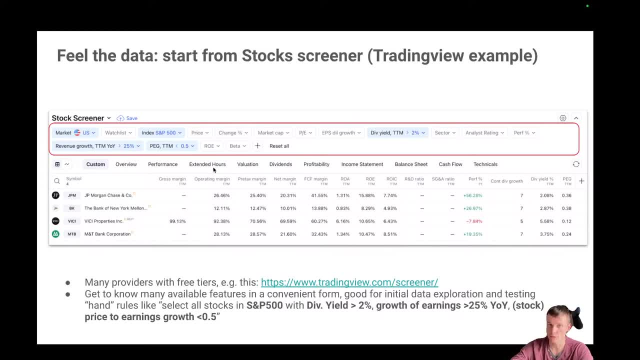 what deputy head, your potential types that you might get. you can see from Here. I designed a simple portfolio with a simple portfolio covered with the Hungarian idea that I want to invest into the US stocks that are included in the S&P 500 program. 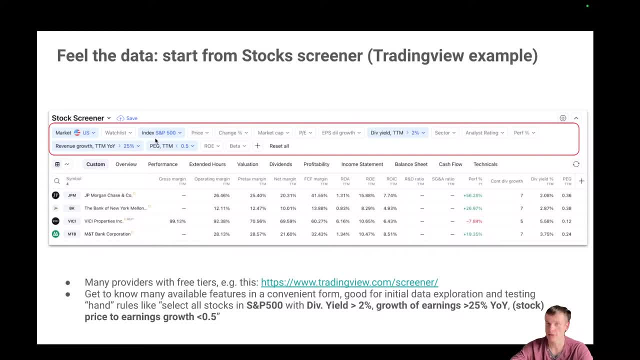 Here. I designed a simple portfolio with a simple idea that I want to invest into the US stocks that are included in the S&P 500 program that have dividend yield more than 2%. I could include other metrics, like biggest market capitalization. 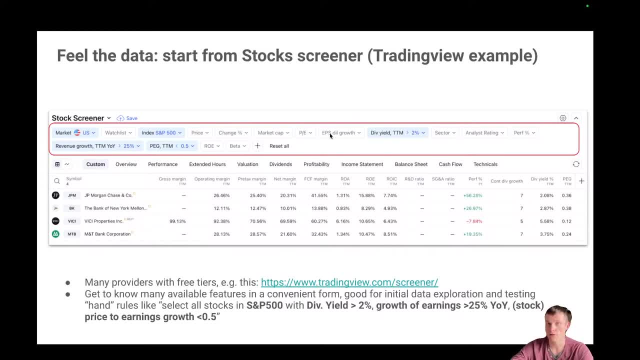 or high or low price on earnings or earnings per share or anything else. And then revenue growth. in the last 25, revenue growth is more than 25% year over year And you can see that it's only for companies within these requirements. 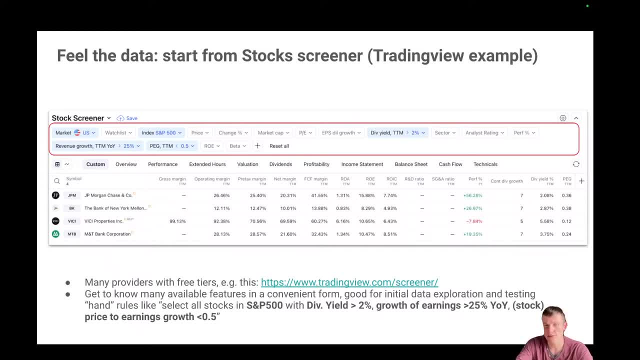 Or if you think about trading strategies- we can discuss it later as a hand rules, Maybe you already know some verticals or some categories and you have these rules when you decide whether you want to invest or not, and you can improve this rule. 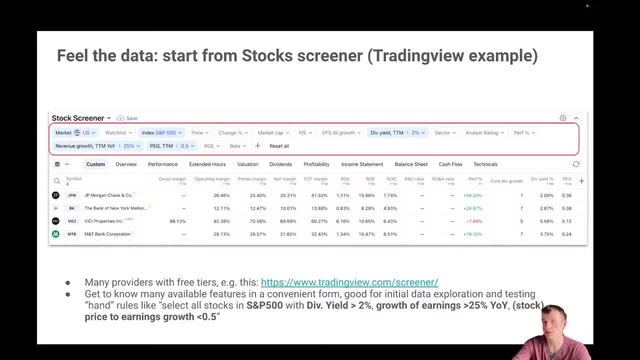 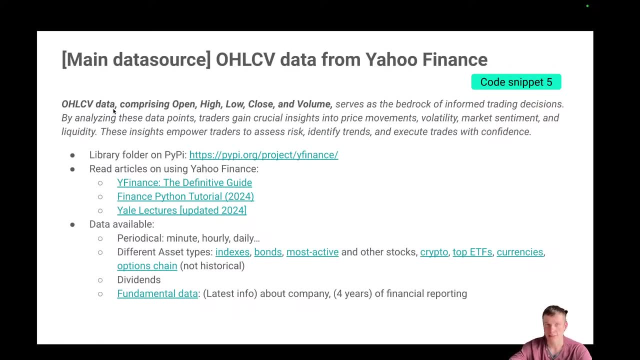 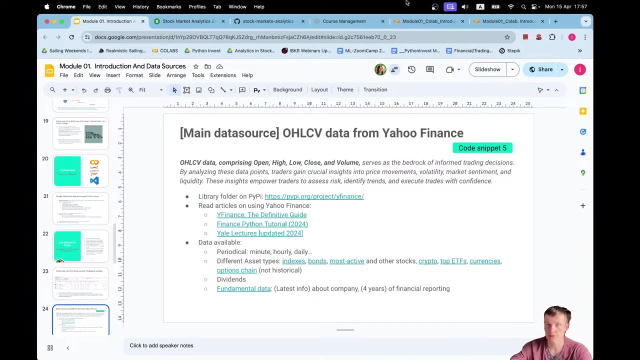 So you can start from these rules before you go into the ML modeling. So this data source, as you can see here, it's the main data source and it is quite an important one. I have more examples here. code snippet five: 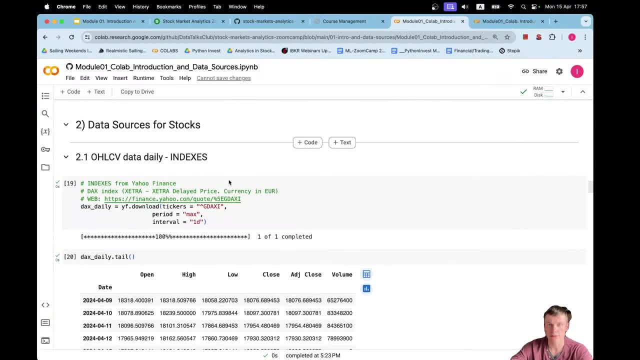 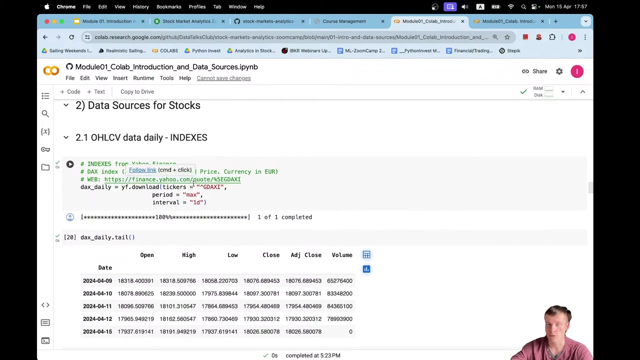 So here you can see that I download data from Yahoo Finance, not from Stook, And you need to read about the description, whether it is a real time or 15 minutes lag, whether it is an index or ETF. For example, if I want to have a DAX German index, 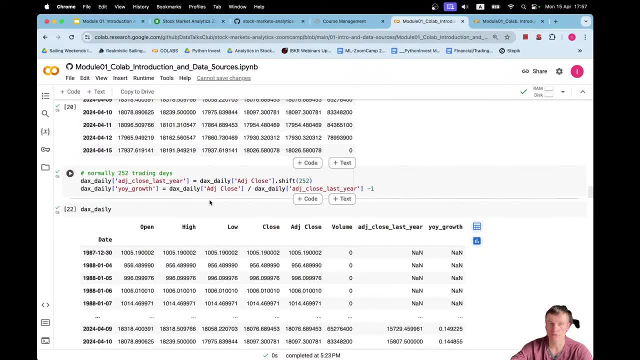 I can get it from here within one line of code. Here is one trick of an approximate year to year growth. As you might know, Stock Exchange doesn't work on Saturdays and Sundays And there are some holidays, So it's quite hard to calculate year over year growth. 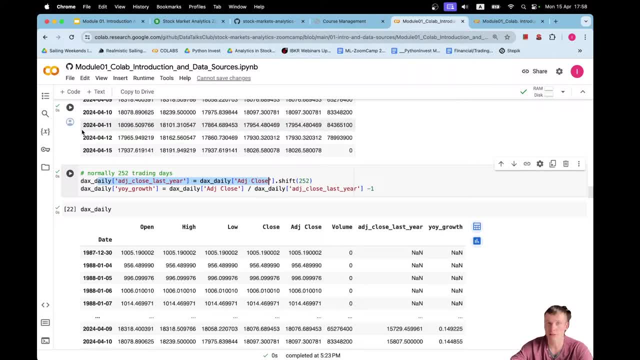 if you just want to match with the date one year ago, because Stock Exchange might not work at that time. That's why we shift on 252 days ago, And it's well known that normally there are 252 trading days in a year. 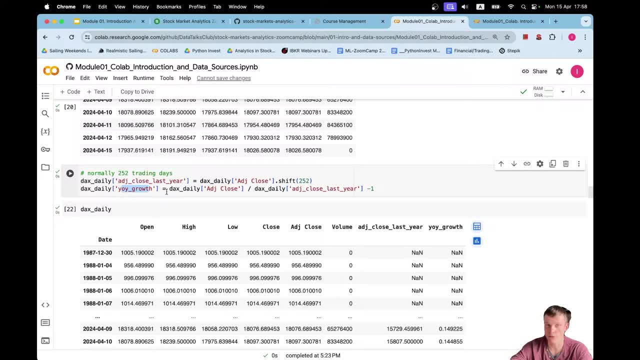 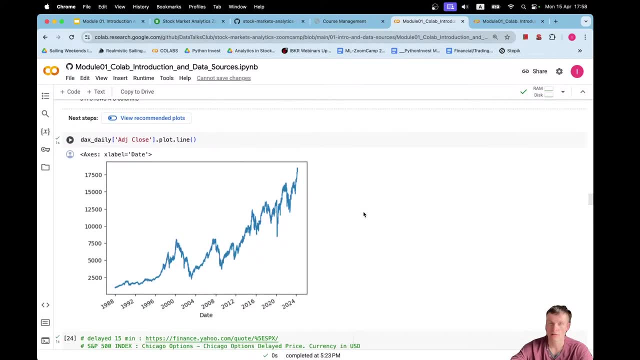 And that's how you can get the year over year growth. We divide adjusted close this year on the adjusted close one year ago. Here is a graph of absolute stats. What I wanted to call out here is that you can select one feature. You can have dot plot and dot line, dot bar, dot area. 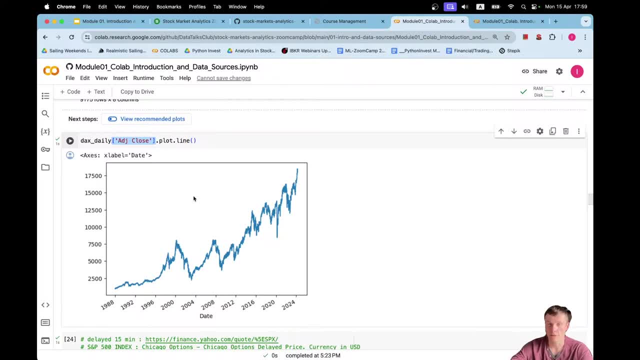 And you can have a visualization. And you can have a visualization without many parameters And when you want to publish it somewhere or prettify, you can ask ChatGPT or you can go and make it pretty. But if you just need to do a quick analysis, 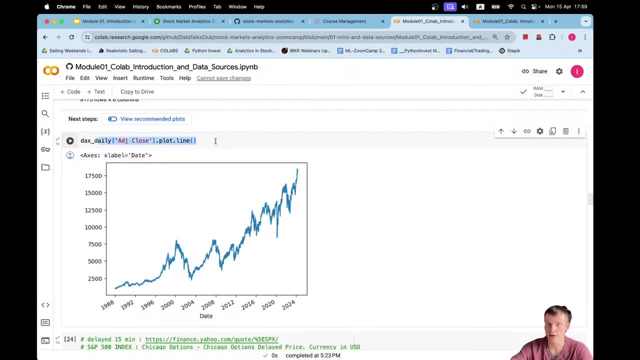 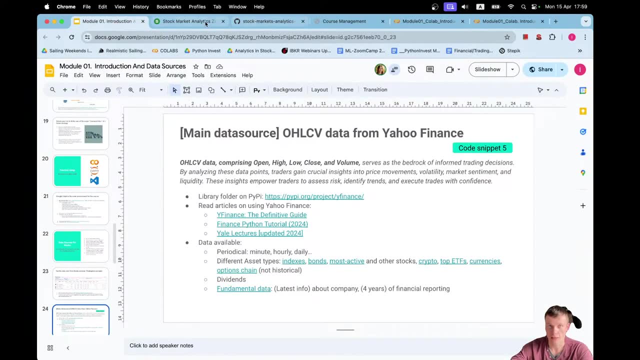 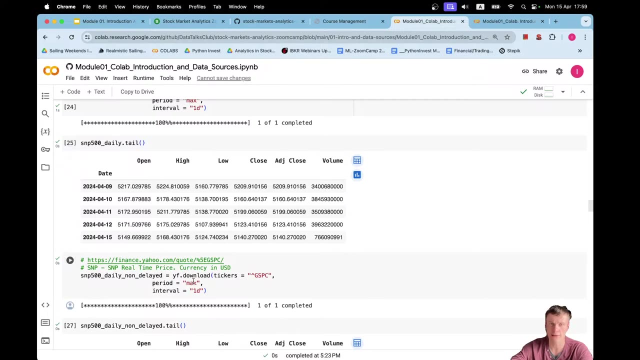 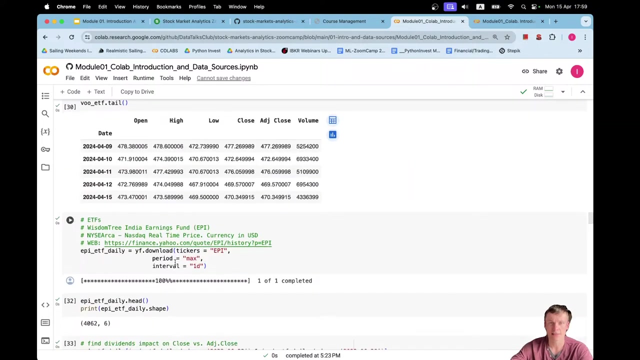 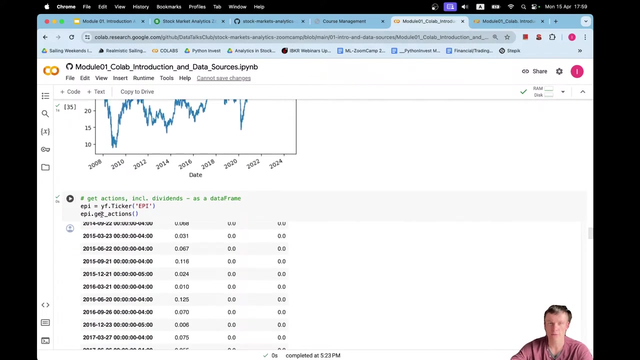 you can be very practical with this one line of code. Okay, What do we have here? S&P 500, daily delayed, not delayed ETFs, other ETFs, So it's all the same. Now we have importance, I think. 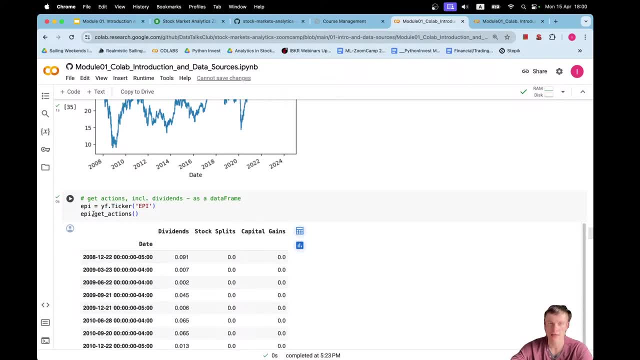 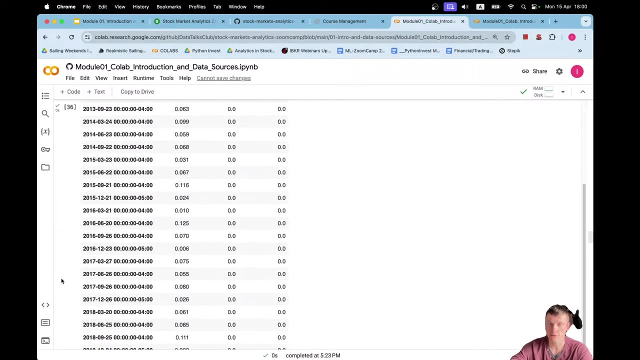 which you need for your home assignments. If you have a ticker- in this case it's EPI- you can use it. You can get actions and you can get dividends with the dates and with the dollars paid as a dividend. So you will be asked to calculate the dividend yield. 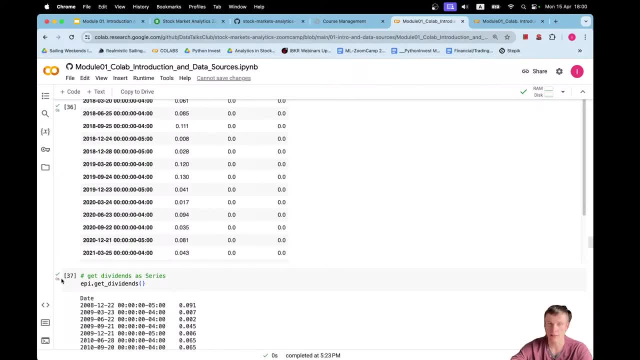 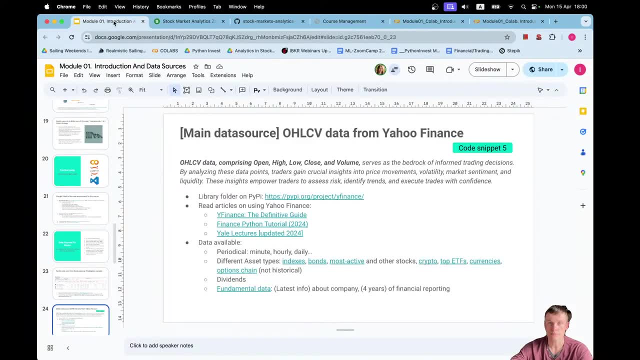 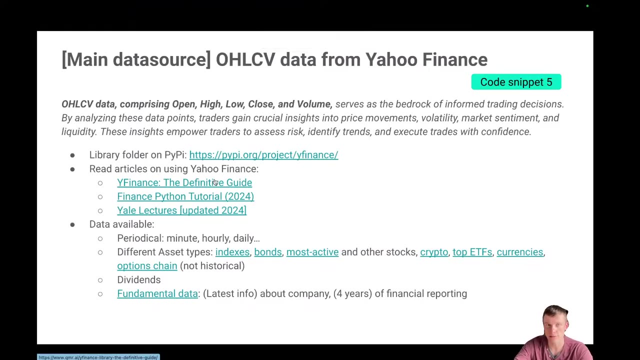 for a particular stocks in your home assignment And you can use these functions. Okay, Let's move on. So please read these articles. You can find more details about the data source. Okay, But it's the most fundamental and underlying data source. 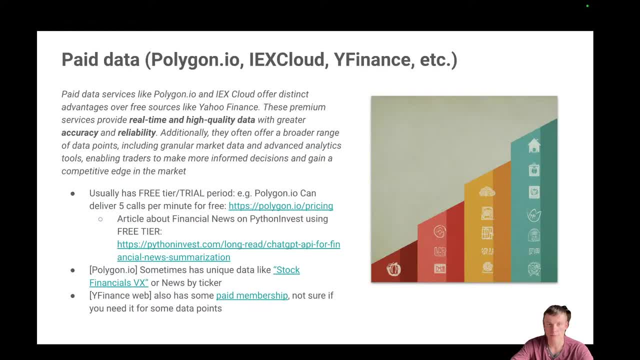 and that we will use everywhere. Next, paid data: I used polygonio. ixclouds, Yfinance has some paid subscription as well. There are some other providers. Please write this in comments If you use them, if you find them useful or better. 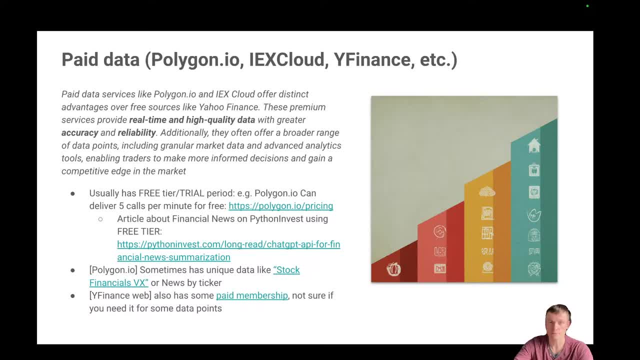 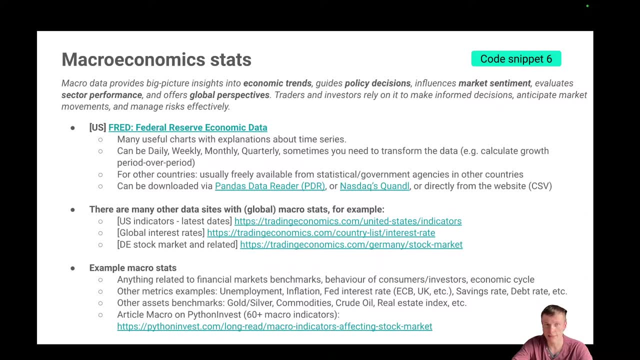 then free data. we can share it with everyone. Let's move on to macroeconomic stats. We talked a lot about FRED and database, but it covers only US data mostly, although it has some global stats. You might want to look at the other indicators. 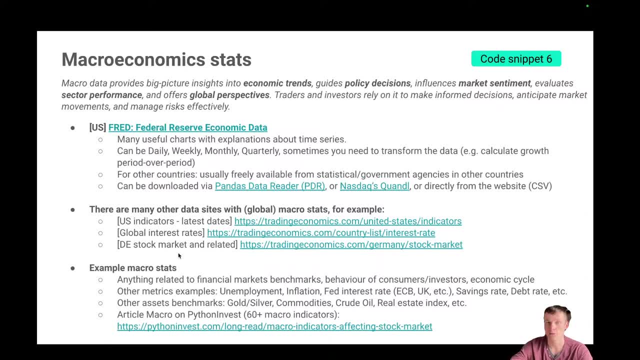 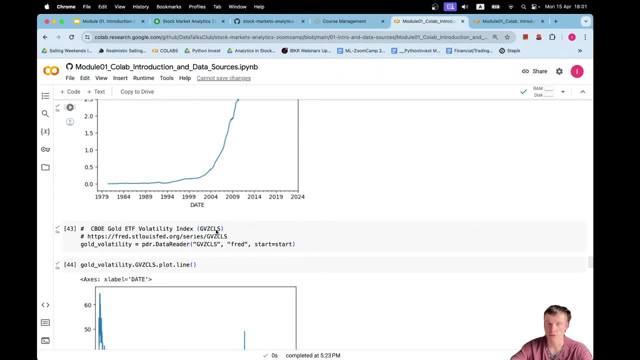 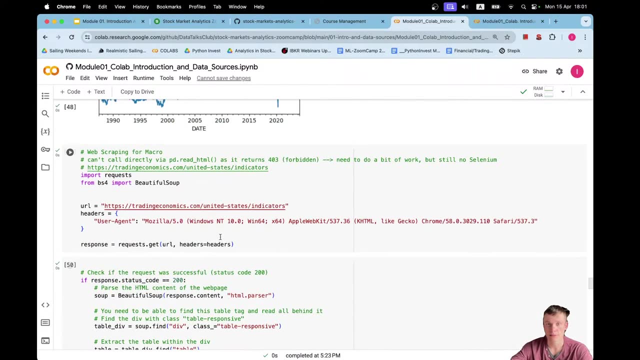 like global interest rates or German stock market and related indicators, And so there are a plant of websites available, and the idea here is that there are here is that you might want to use web scraping, or they can have their own subscription and provide the data via API. So here, for example, I have URL. 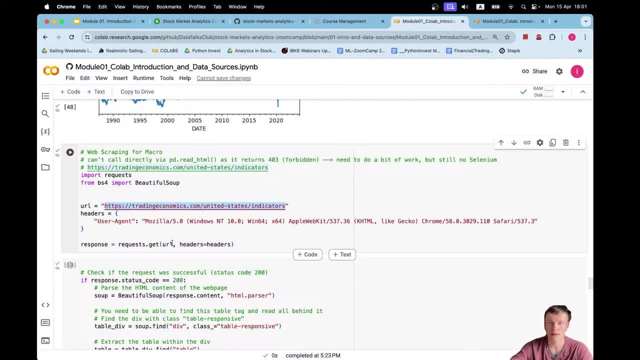 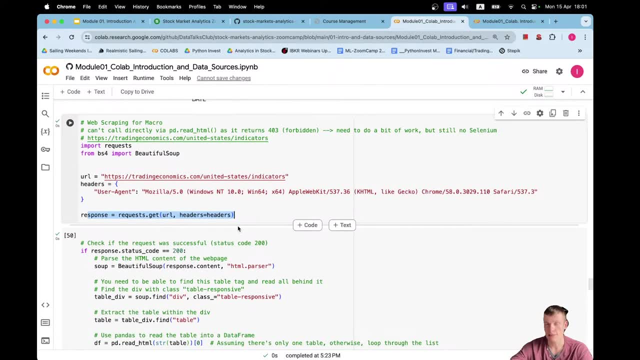 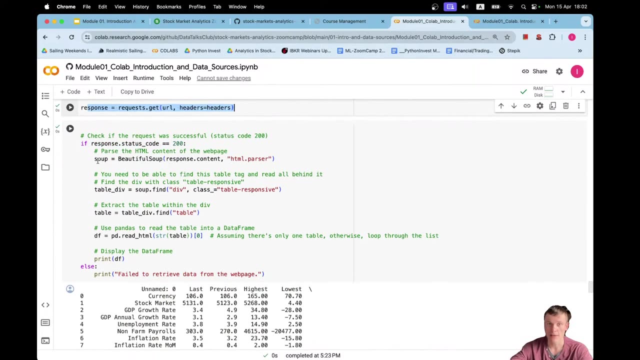 trading economics: United States indicators- standard headers. I write this requestget and in many cases, for the static web page, you will receive some some response and then you can find specific elements. In my case it's a table, so you need to know a little bit about HTML markup, but you can also ask. 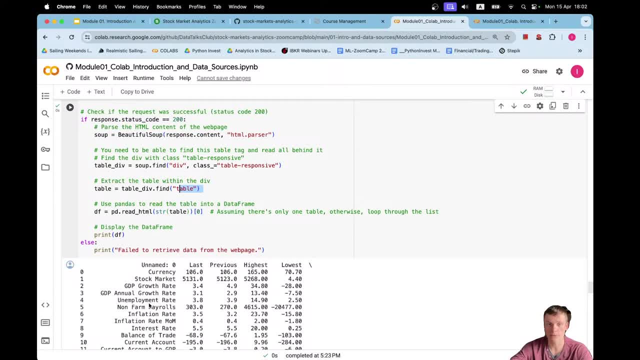 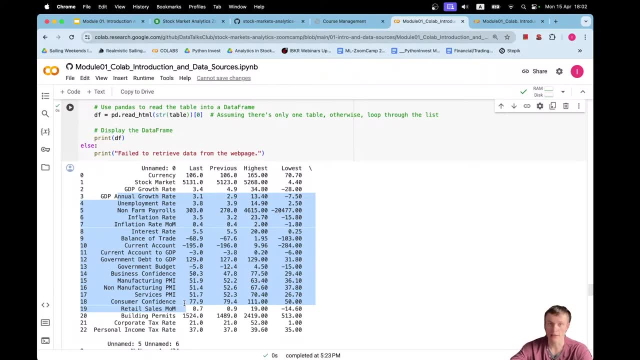 ChatGPT and it can provide you a working code. And that's now. you can see that there are many metrics available via web scraping and also with a screen reader. China is also very famous for its web-basedunuities and the comparing南ка page of the Russian external world. in the world of 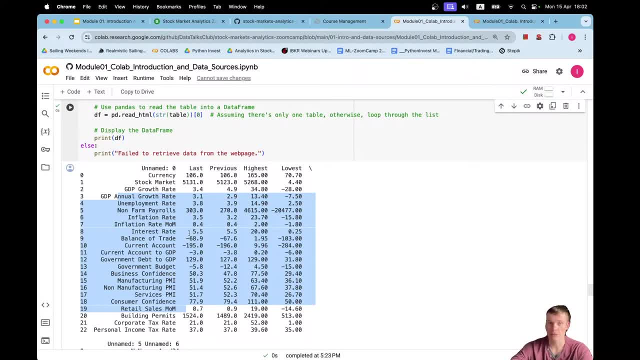 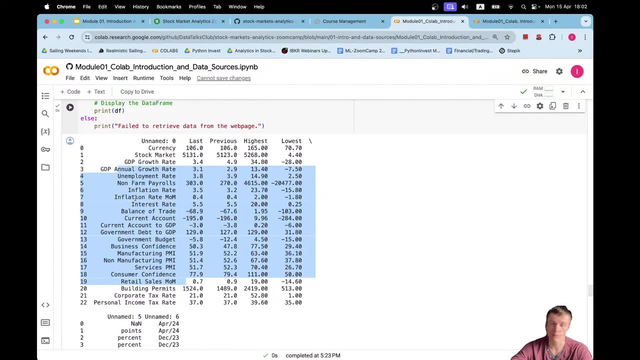 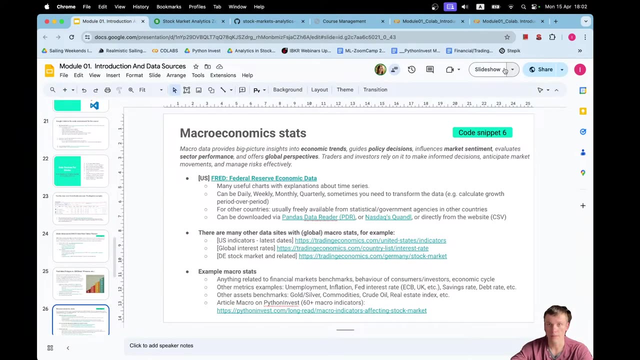 and the other way. here the back-end is not on Americanンド and we don't use that information topic for our videos, but there are performance value projects. The problem is that there is no historical stats for all of these metrics, But you can find separate pages for each of the metrics and they might track it. 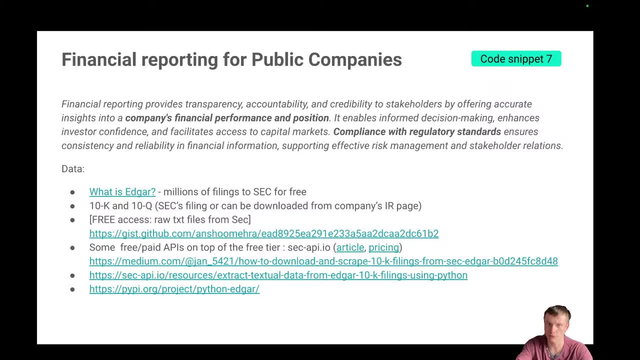 Financial reporting for public companies. I think about 30-40 years ago there was a system called AdGuard- millions of files there. So if you are a good software engineer and you want to build a system using local or hosted LLMs to analyze those feelings, I think it is very good thing to have. 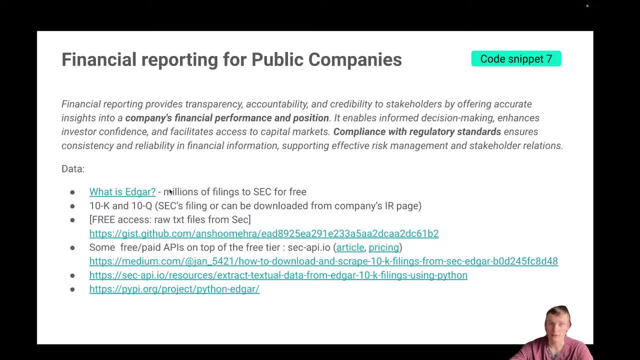 It's hard but possible. You can download these raw text files. You can analyze them. There are some paid products. Companies like sec-apiio provides access to the data and they have some free tiers of probably first 100 calls that you can do for free for you. 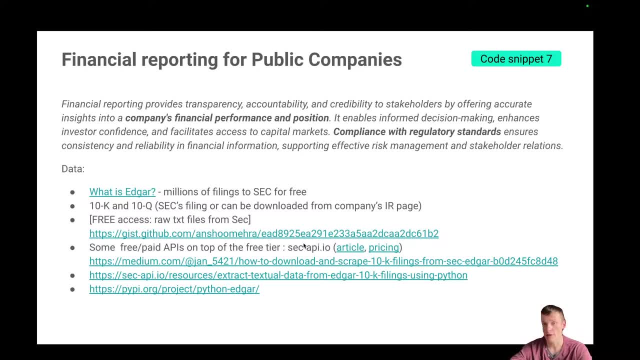 So they already downloaded the data, wrapped it in a Python package and made it available for you to be used. But the downside? The downside is that oftentimes it is paid, And there are some other examples how you can use this data as well. 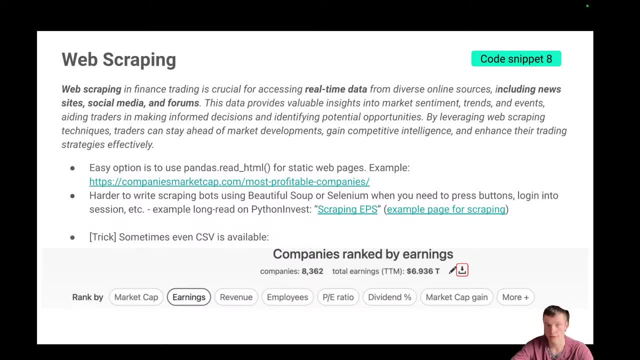 Web scraping. I already showed how you can do this. I think it's a very powerful thing. especially, you can replicate or replace those market screeners just within a few, maybe hundreds lines of code. For example, This website: companies market cap. 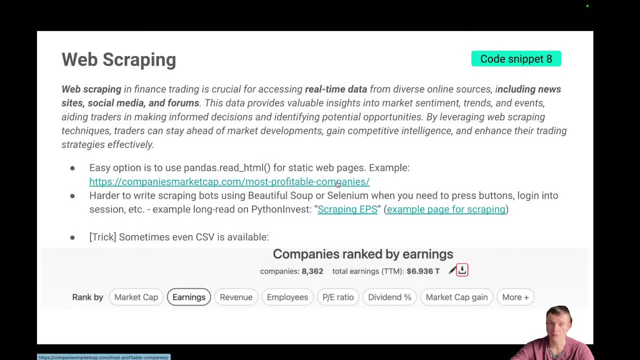 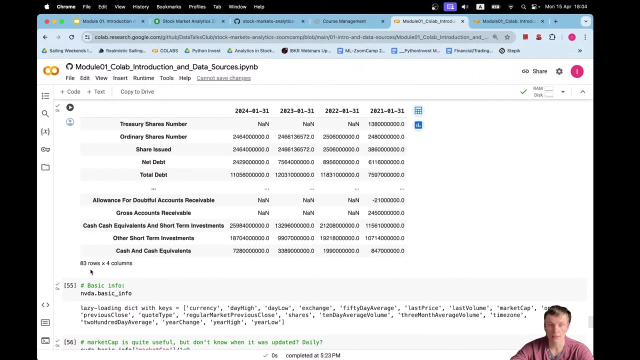 It has different pages, like most profitable companies, on earnings, market cap, revenue, employees P ratio and many of these pages. They have a download CSV file button and you can see in this code, snippet number eight. That's you can. You can download this, this file, very easily. 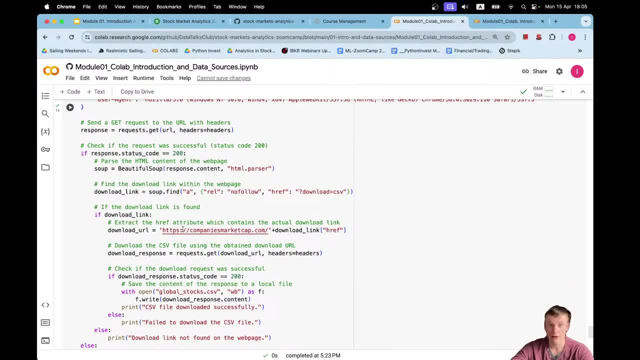 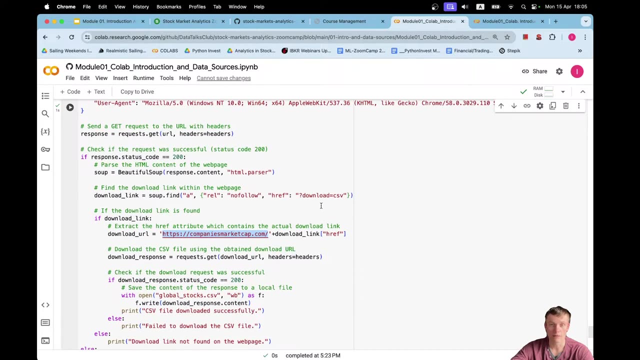 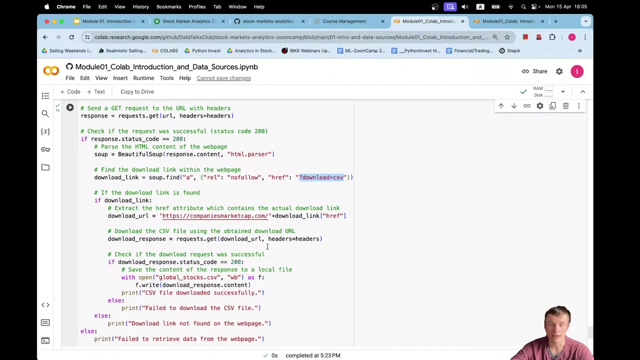 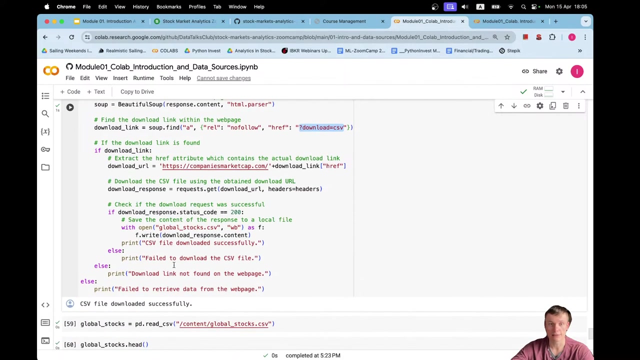 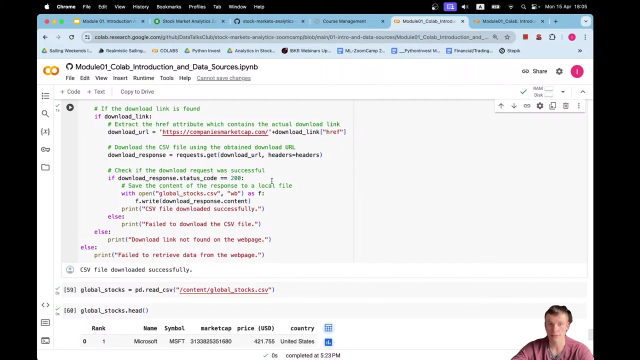 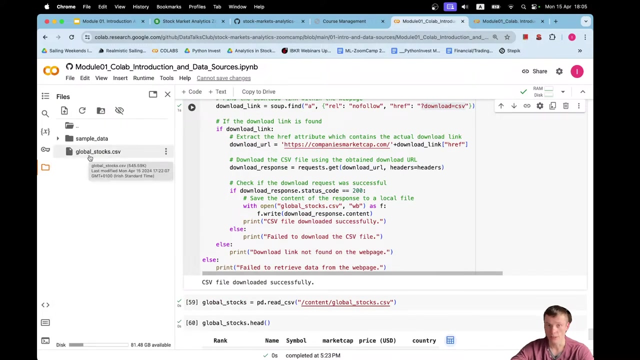 There is a URL and then I have downloads, download link with these parameters: download equals CSV. I saved it. I saved it. I saved the response in the text, I write it to the file and I read it from CSV. So, as a result of this call, I have CSV file generated, which, which is a file that was. 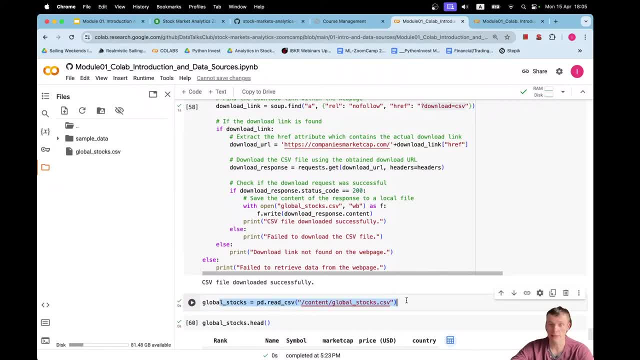 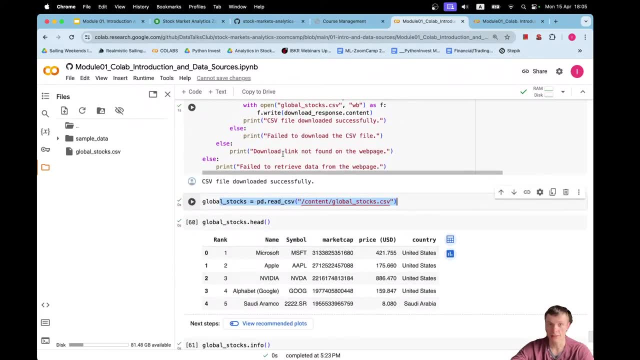 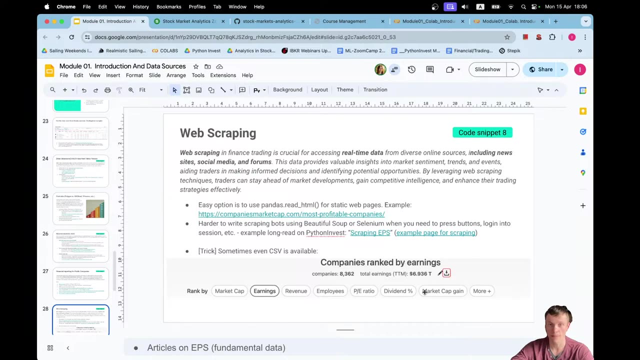 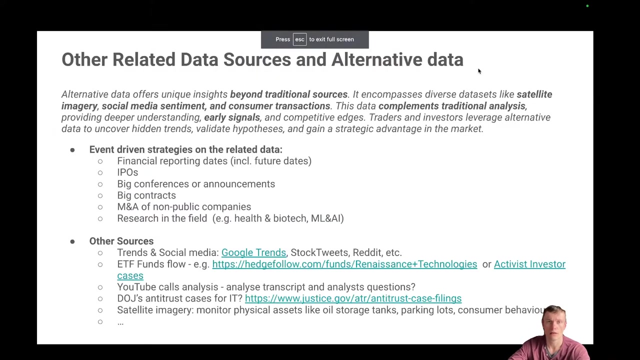 downloaded from the, from the website, Then I read it with pandas And now I can analyze all of this, All of these data, and actually that file contains information about 8000 stocks straightaway. So you see 8362 companies. Financial news. 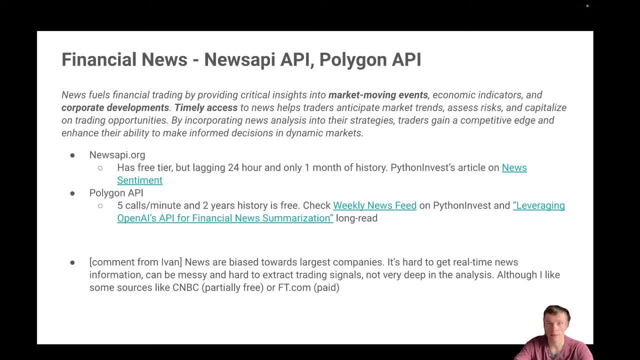 I don't have examples straight away. It's quite, quite hard, For example, for for for a retail investor to build an efficient trading strategy around this, probably because news are centered around largest companies. you will get them after the reporting is published or after a few days of the event, and 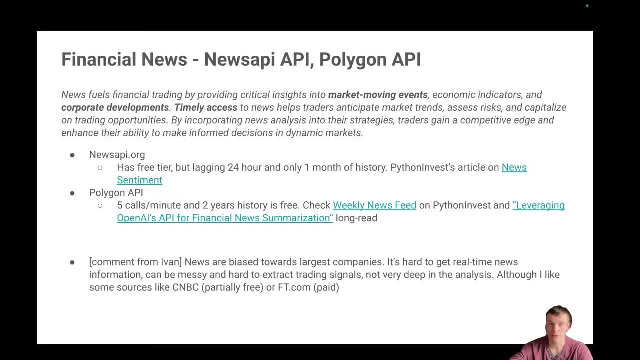 probably it is too late and oftentimes they are built by journalists and not financial analysts, so you might create a better analysis by yourself, but I tried to to do some analysis on use and there are two articles on the Python invest website. it's one is on new sentiment and news API and second one on polygon dot. 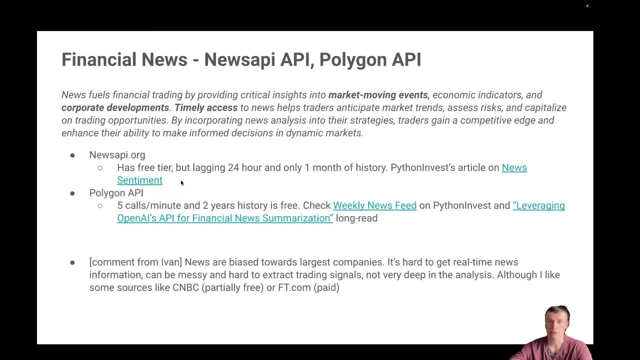 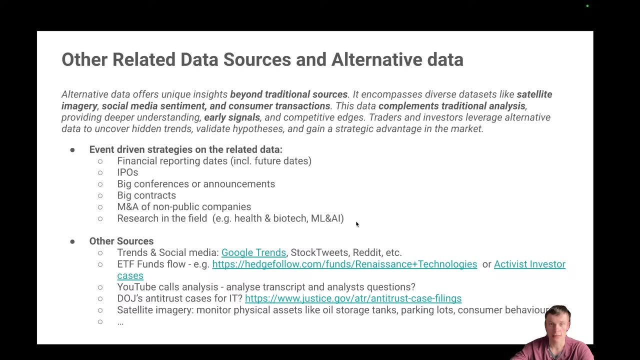 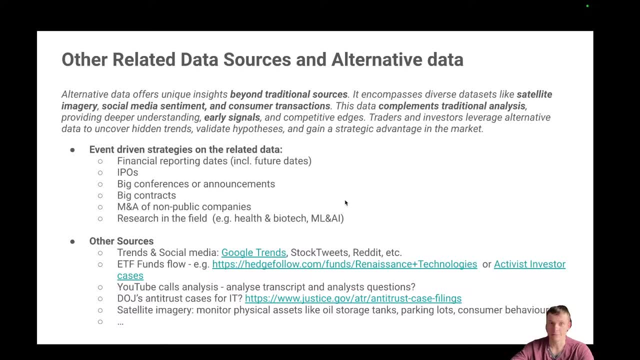 traditional sources, for example financial reporting dates, you you can anticipate future reporting dates or companies that you are tracking and you can track straight away and download the reporting information. or YouTube screencast- just minutes or even real time, when it have it happens and do the trading, Then IPOs. you may know when new companies will go. 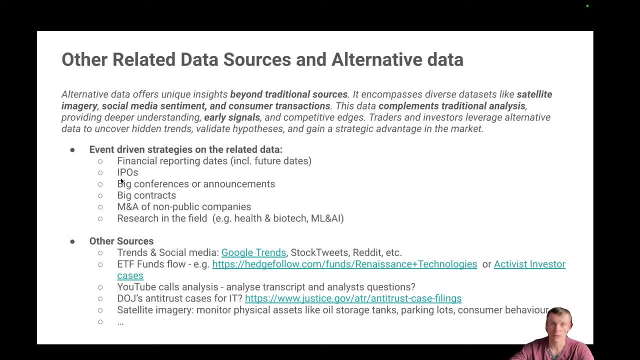 into IPOs. you can build a model to predict whether that IPO will be a long-term growth or not. Big conferences and announcements: I'm working for Google- many IT companies. they announce new products or new model shipments at their conferences and it can actually change their stock price just after. 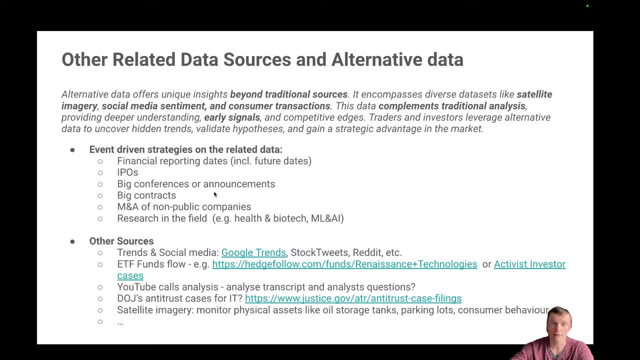 the announcements, Big contracts. if you can have a proxy for a new big customer, that's a good thing. to have Merchants and acquisitions of non-public companies, Very often even public companies. they grow when they acquire smaller non-public companies, whether they 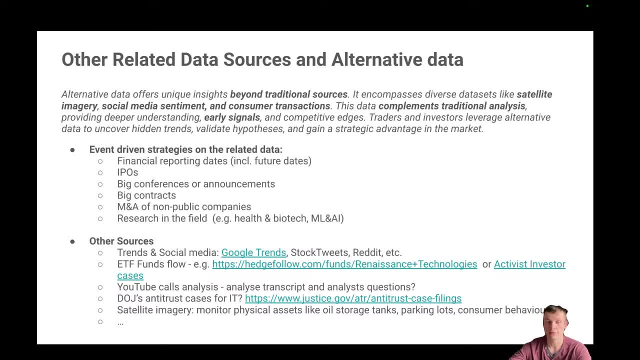 acquire some product or some team and if you read about it, you can trade respectively. Then research in the field. There are articles on machine learning and AI, health and biotech. There are experiments so you can track who is publishing them and whether the 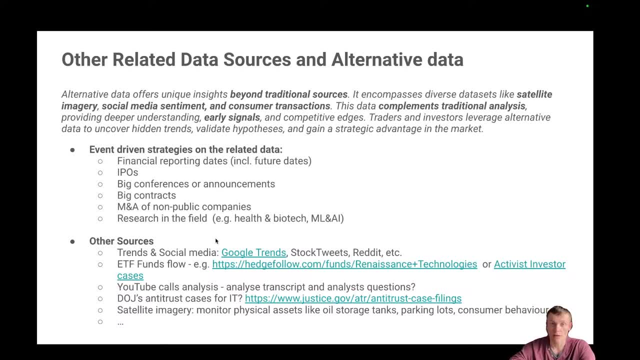 amount of articles can predict the stock prices. Other sources: trends on social media. I think it's quite messy: Google Trends, Stock Tweets, Reddit. Probably you can generate something meaningful. ETF funds flow. There is a website, hedgefollowcom, and you can track your funds of interest, For example, Renaissance. 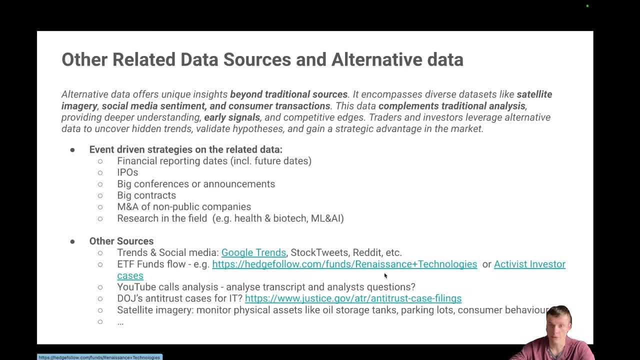 Technologies that has a very good long-term performance. You can see what do they currently have or activist investor cases, top funds. Then you can download YouTube calls- YouTube videos with revenue calls- and check the information shared there. I think what is heavily under-researched is questions from analysts and the responses from 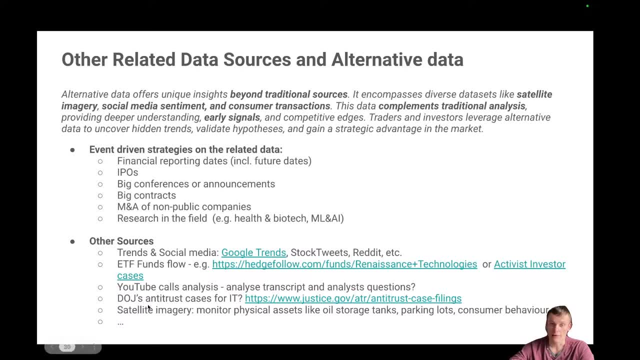 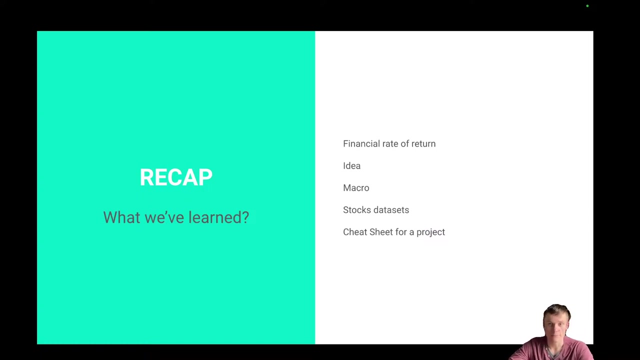 from the management For IT, for big tech companies and Department of Justice. antitrust cases is becoming quite an important thing because there can be fines on those companies. Satellite imaginary You can. you can come with many more sources. Think about it. Recap What we've learned today. We started from a concept of 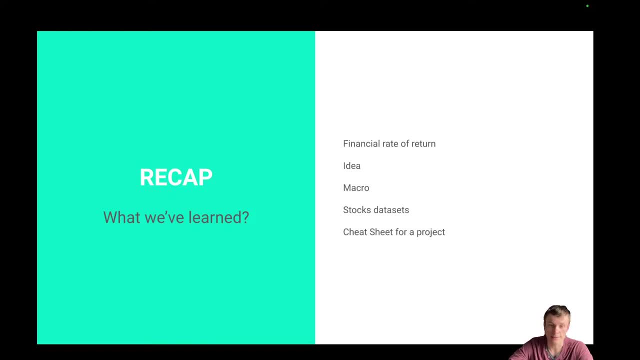 financial rate of return if you just save money as a retail investor, if you, if you try to invest into into the saving accounts, into the bond market, into the stocks with a passive strategy, then we came up with with the idea that you need to have some benchmark and 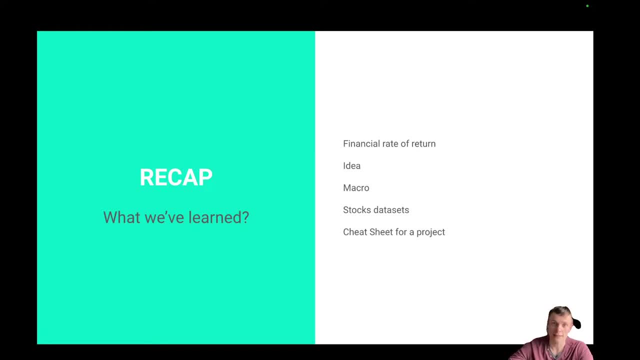 and compare your future trading strategy with with this benchmark. so you will want to develop a future strategy good enough to be more profitable than a benchmark in most of the times. then we talked about many macro data sets or the data time series. we discussed some of the stocks and data sets and now we will 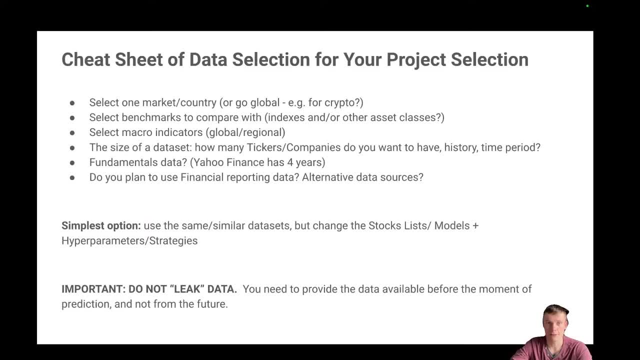 have a cheat sheet for project. so if you, if you think that it's it's too much for you, if you just started doing all of that and straight away, i share you the the knowledge and information that i captured over the period of three years. you just need to do these, these steps, and probably you, you can just replicate most. 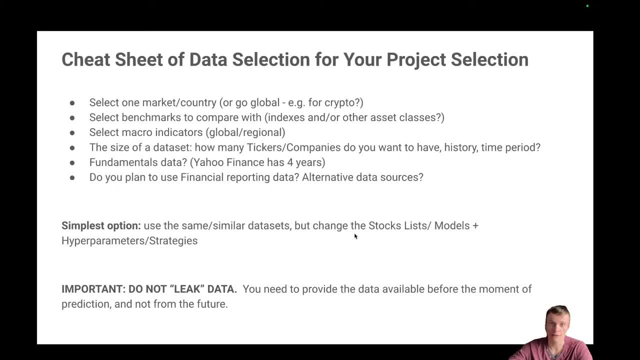 of the steps that they have, and you don't need to change a different vertical or or step markets. you can just work on exactly the same data but change slightly with the companies that that you use or with the approaches, with the models. so what i would advise you to do when you are thinking about 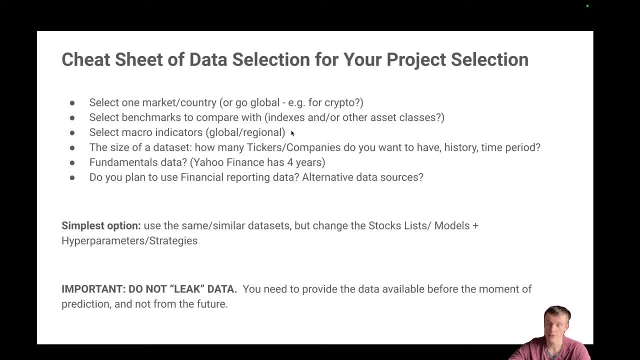 your project and actually there was a good question in in slack that if, if i can start working on your project, i advise you to start straight away, right now, to work on on your project, because this is the most important thing for you and to have as a result of this course. i would advise you to select one market or country. 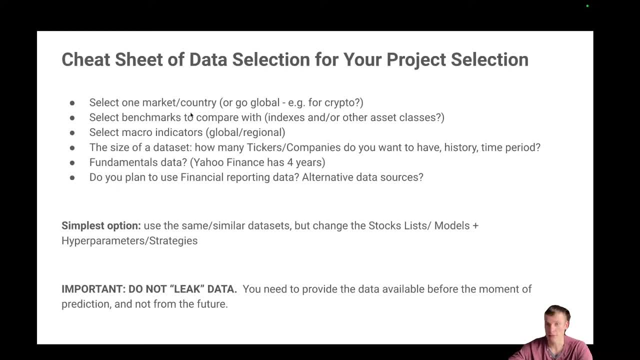 i don't think that stocks- that global stock strategy is- is an easy thing to do. probably, if you do for a crypto, you can go global. then select benchmarks to compare with your risk return profile- something that you see oftentimes in the news- and you compare against. 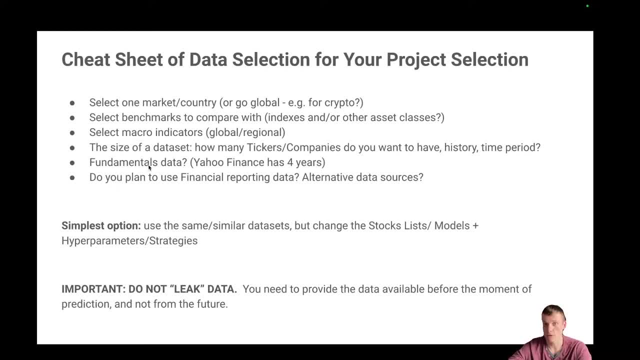 select some macro indicators or economic context that you have it. it may be global, it may be regional, it may be your, your country or the. actually, i advise to to compare versus options that you currently have and that you have currently in your portfolio, versus options that you currently have and that you have currently in your portfolio. 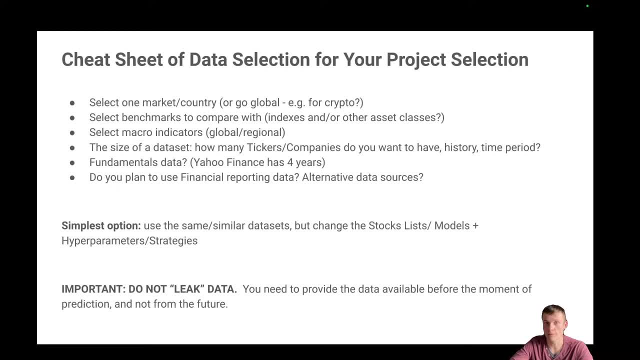 have to save and what is the most impactful thing for your personal saving and investments and spending decisions. then you might want to think about the size of the data set. how many tickers companies do you want to have? I try to to have 250 companies from from the US and it was a three million records data. 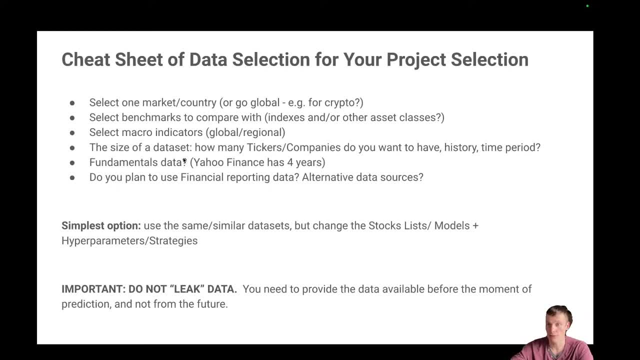 set with 300 features generated and it was a little bit too heavy for pandas. so probably you you will want to start from a smaller data set, but you need to think about it: fundamentals data- where to get it? for how long Yahoo finance provides data for for the last four years? do you plan to build something in around 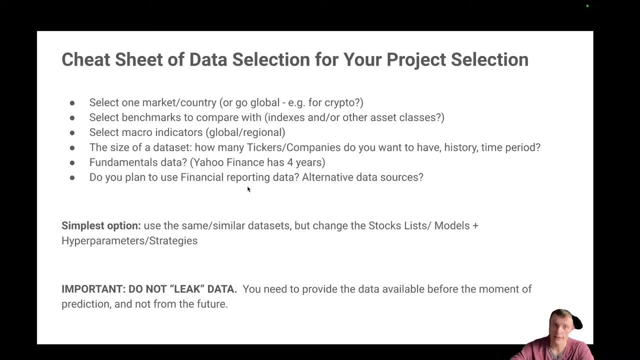 financial reporting data. whether you want to analyze large- you want to analyze large amount of text or not- whether you want to use alternative data sources, the simplest option is to use same or similar data sets, change stocks, list models, hyper parameters and strategies and build something for for yourself one. 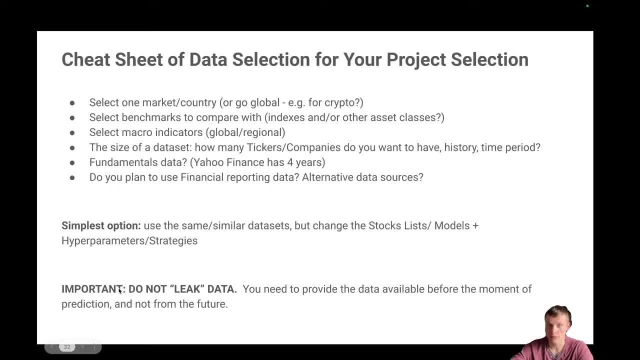 thing that's that I want to caution you is: do not leak the data. the thing is that you you need to think what is available at that moment of time. if you generate some data that's that was available one year ago, you can't include any future known features, because 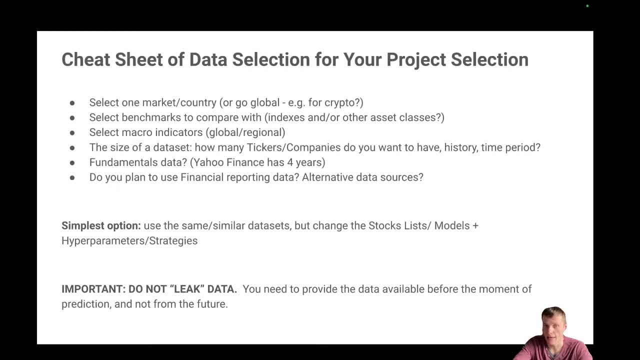 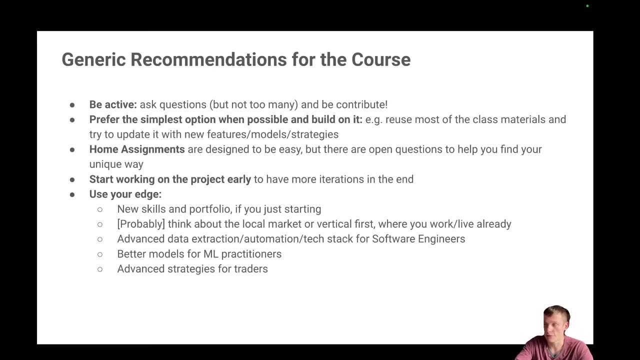 any model will quickly capture that and it will bias the results. you won't be able to trade and to use that information and some generic recommendations for the course. this is designed to be free for everyone and please be active and helpful. ask questions. ask questions to the slido on a telegram. reply to questions on on slack. if you know the answer, I would. 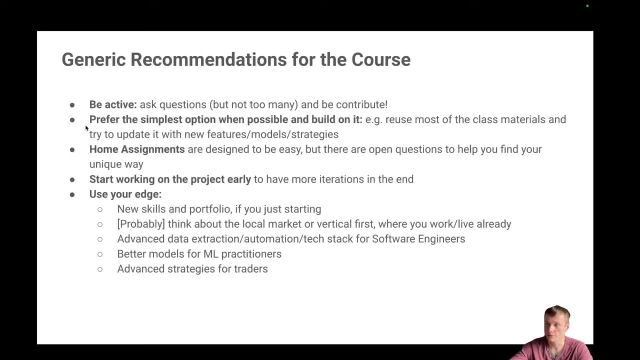 advise to prefer the simplest option when possible and build on it. so you you need to iterate quickly. I would just say that reuse most of the class materials, try to update with new features, model strategies, and you are asked to do this with two questions in the home assignment. 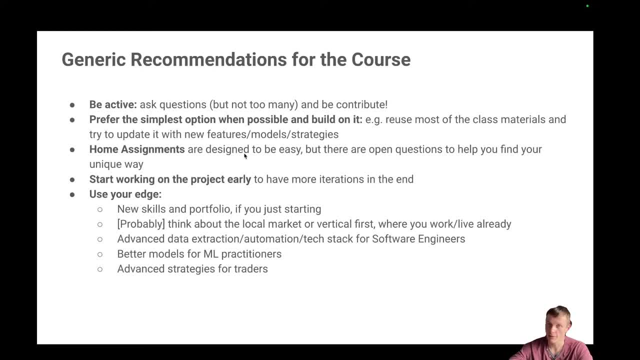 home assignments designed to be easy, but there are questions for exploration. no, it may be not always easy, but they are straightforward. there are no tricky questions. start working on the project early and use your edge. so, if you're an analyst or just build analytical model, and use your analytical skills if, if you 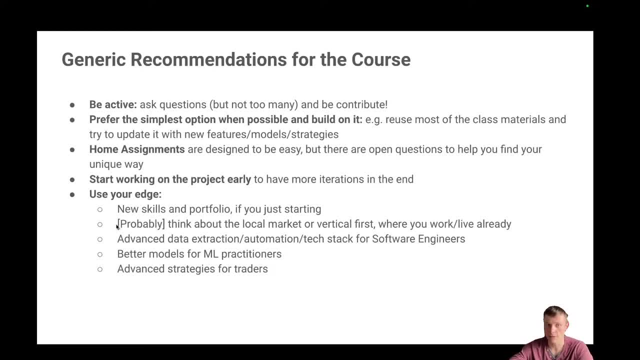 leave and you know a lot about your, your country and some specific market where you work in. just go and build a model around this country and market. that's how you might see less competition and you have better knowledge. if you're a software engineer, you might use advanced data extraction automation tech stack for your models. if you're a ML practitioner, 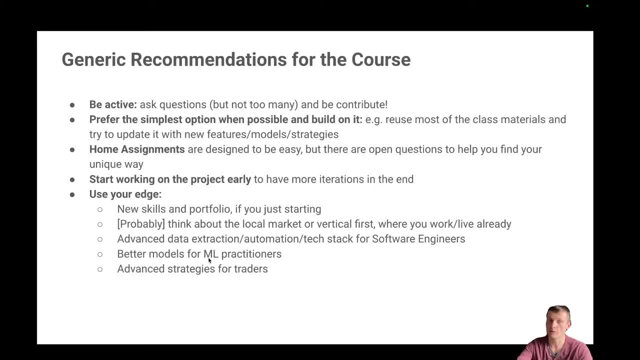 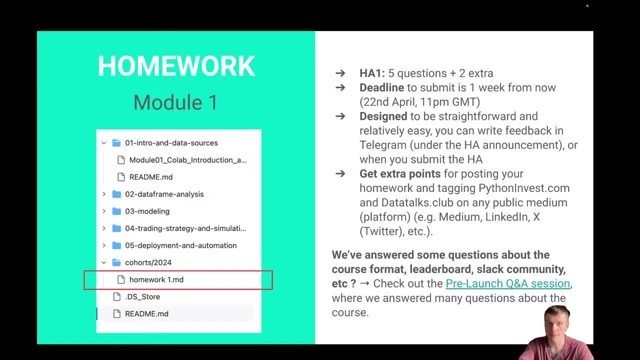 ML engineer. just go and build a more complicated ML model and probably you will get better results. homework: you might have seen that homework is already published. it's in cohorts slash 2024, homework onemd. you can already submit the homework. there are five questions and two extra. it looks like this: 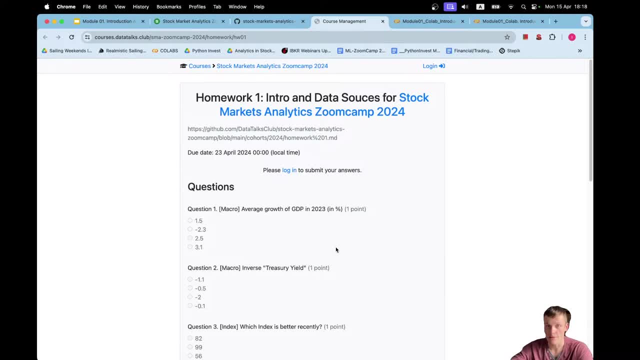 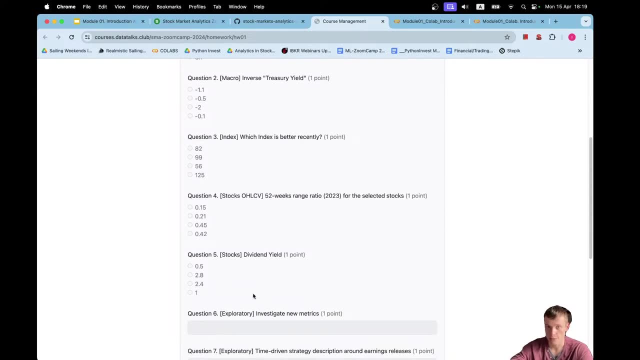 um. so there are questions and there are numerical answers: question one, two, three, four, five. please use the code that that I shared you. you can find most of its um in most of the examples that you need in the code um. then there are two open-ended questions: exploratory- investigate new metrics- from the same. 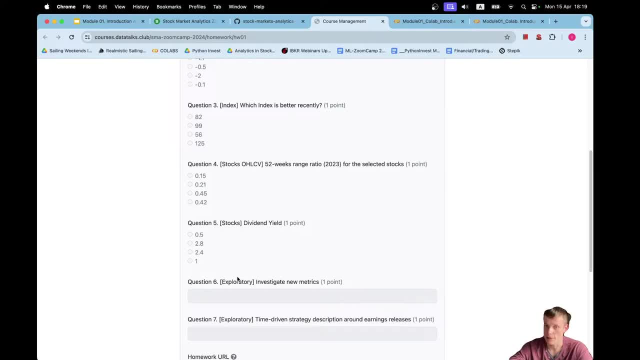 data sources and try to read articles about it and briefly explain why are you doing this. and then another thing to think and to design a strategy, a time-driven strategy, around earnings releases. Let's assume that there is an active earnings releases season and you want to build something around it. You don't need to. 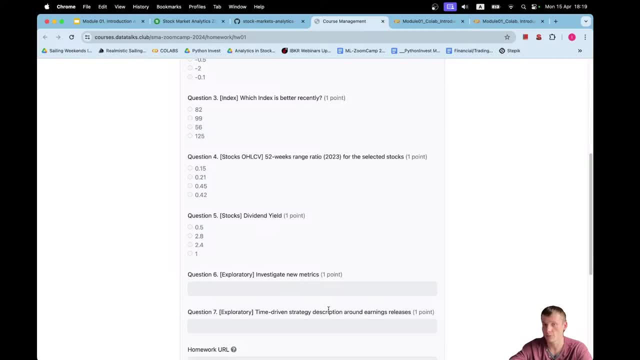 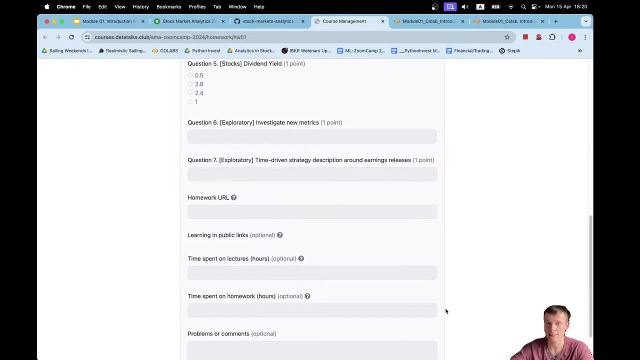 implement it. but just explain here, while you don't know all the details, how to do their modeling and simulation, Try to show how to build their end product product on this And there are some standard links on standard questions from any Datatox club homework assignment and you will need to supply.